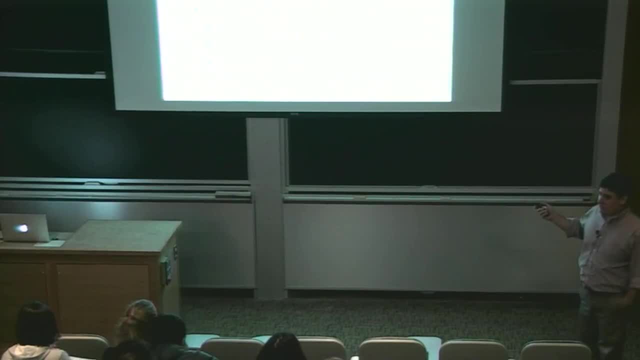 time for the quiz is 7 to 9 pm. We really did try hard to get the scheduling office to give us something better, but the only way to get a room that would fit everybody in was to do it at this time in Walker. I really don't understand, because I actually 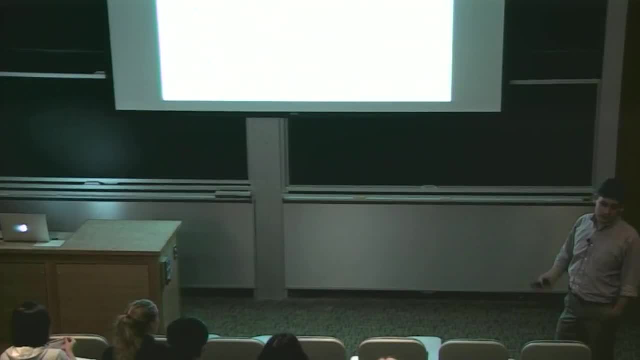 requested locations for the quizzes back in April and somehow, I don't know, I don't know. I was, I don't know, too early maybe and got buried under a pile. Maybe not important enough, I don't know. but it's going to be from 7 to 9 next Wednesday, right, Third floor. 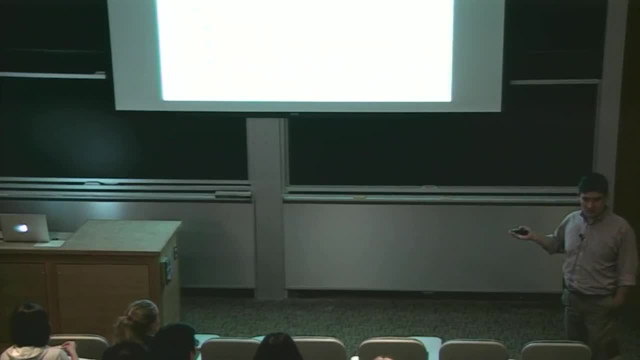 There's not going to be any class next Wednesday because you have a quiz instead, so you can get a little extra time to relax or study, prepare, calm yourself before you go into the exam. There's no homework this week, Okay, So you can just use this time to focus on. 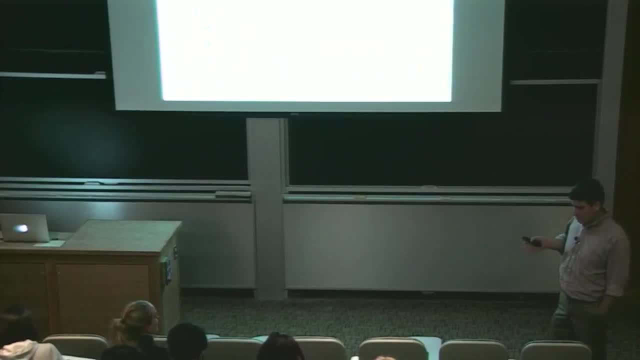 the material we've discussed, There's a practice exam from last year posted on the STELR site which you can utilize and study from. I'll tell you this: That practice exam is skewed a little more towards some chemical engineering problems that motivate the numerics. I've found in the past that 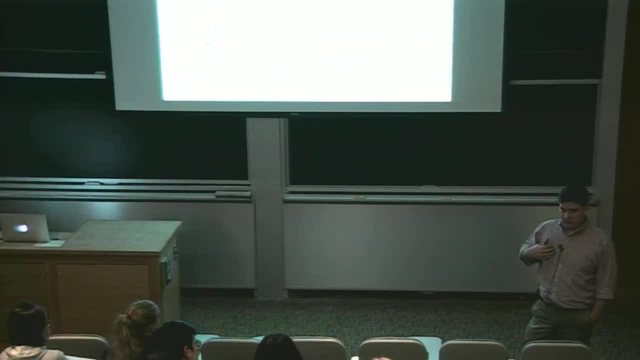 when problems like that are given on the exam, sometimes there's a lot of reading that goes into it- understanding the engineering problem- and that tends to set back the problem solving. So I'll tell you that the quiz that you'll take on Wednesday will have. 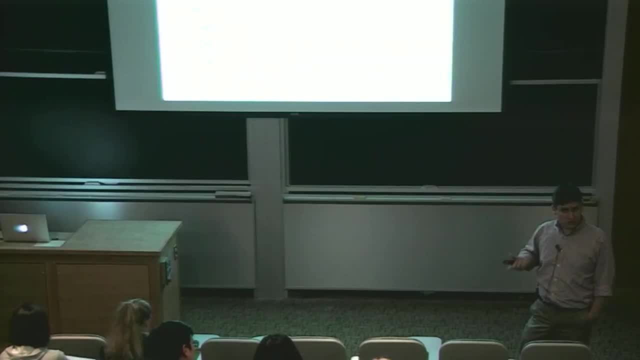 less of the engineering associated with it and focus more on the numerical or computational science. The underlying sorts of questions, the way the questions are asked, the kinds of responses you're expected to give, I'd say, are very similar, but we've tried to tune the exam so that it'll be less of a 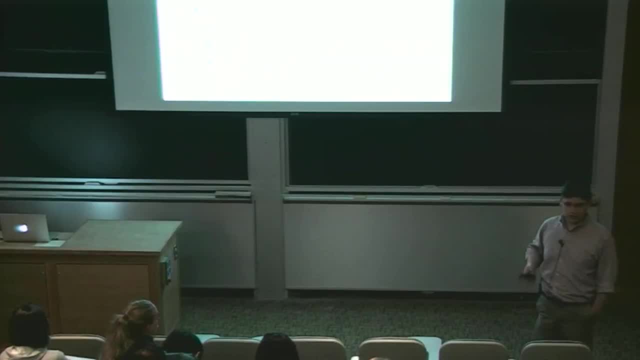 burden to understand the structure of the problem before describing how you'd solve it. I think that's good. It's comprehensive up to today. So linear algebra, systems of nonlinear equations and optimization are the quiz topics. We're gonna switch on Friday to ordinary differential equations and initial 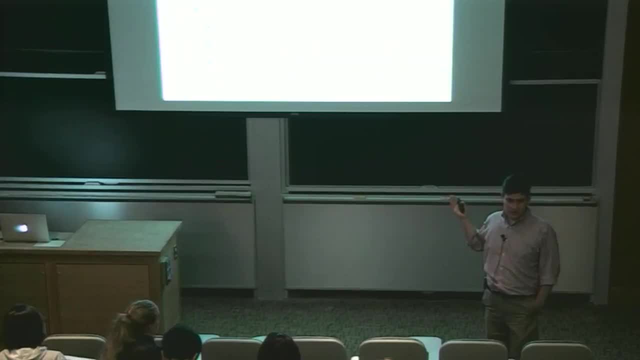 value problems. So you have two lectures on that, but you won't have done any homework. You probably don't know enough or aren't practiced enough to answer them, So I'll let you do that. I don't want to answer any questions intelligently on the quiz, so don't. 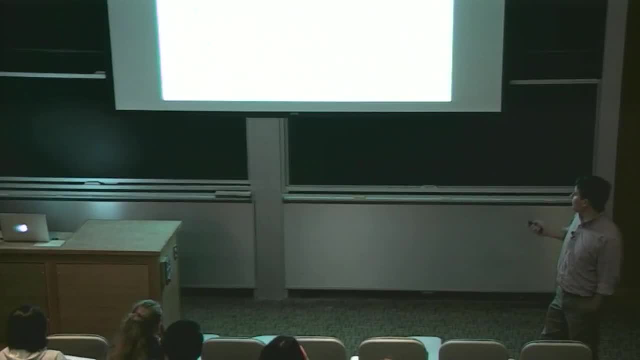 expect that material to be on there. It's not right. It's gonna be these three topics. Are there any questions about this that I can answer? Krista, I just wanted to comment that the WACC Memorial is not the best campus for regulation and how you're going to explore it if it's cold or if it's hot. it's not ideal. 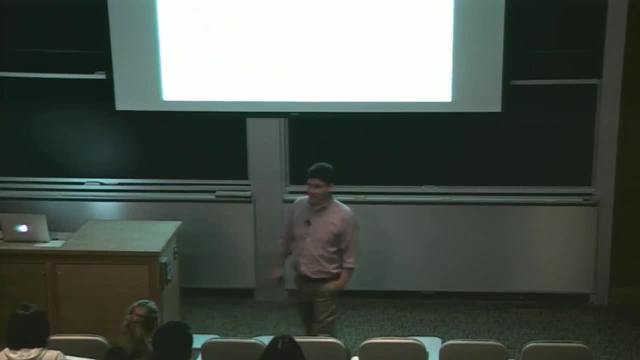 Okay. so yeah, come back next week, Come prepared. it might be cold, it might be hot, It leaks when it rains a little bit. Yeah, it's not the not the greatest spot, so come, come prepared. That's true. 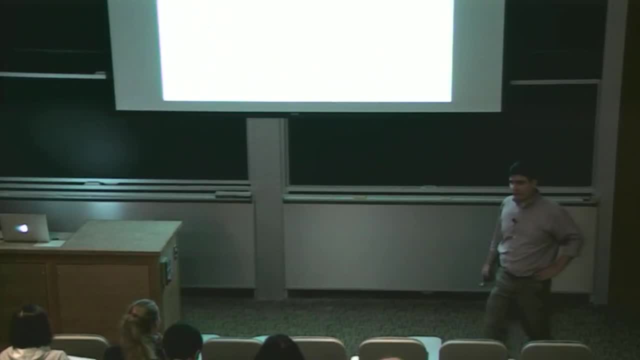 Other questions, Things you want to know. Ooh, good question. so you can bring the book recommended for the course. you can bring your notes. you can bring in a calculator. you need to bring some pencils. We'll provide blue books for you. okay, to write your solutions. 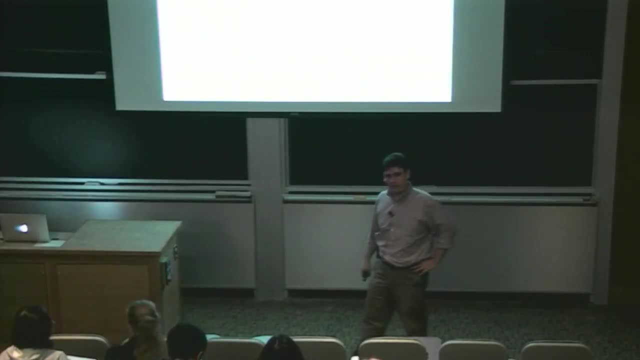 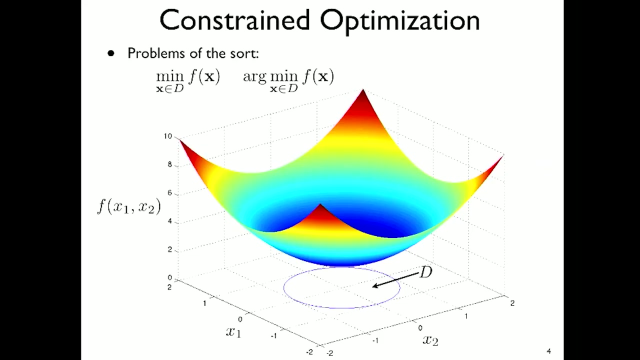 to the exam in. So those are the materials, Good. What else? Same question: Okay. Other questions: No, Okay. So then let's jump into the topic of the day, which is constrained optimization. Okay. So these are problems of the sort right. Minimize an objective function. f of x, subject to the 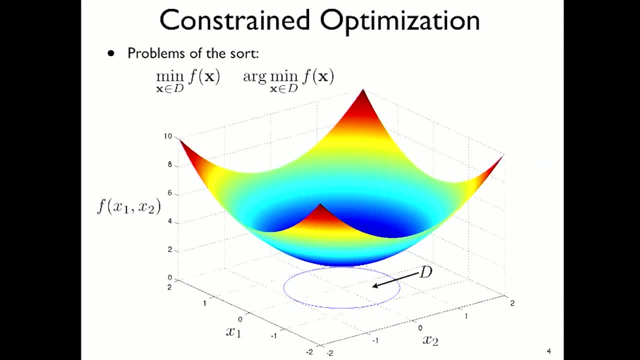 constraint right that x belongs to some, set d, or find the argument x that minimizes this function. These are equivalent sorts of problems. Sometimes we want to know one or the other, or both. That's not a problem. Okay, And graphically it looks like this: Here's f, our objective function. 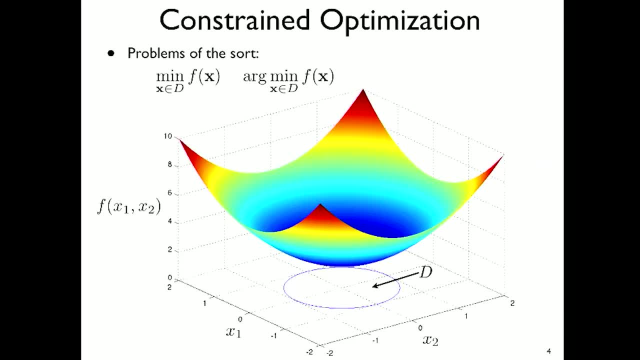 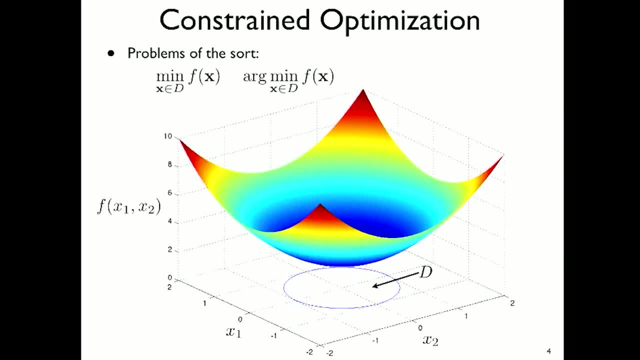 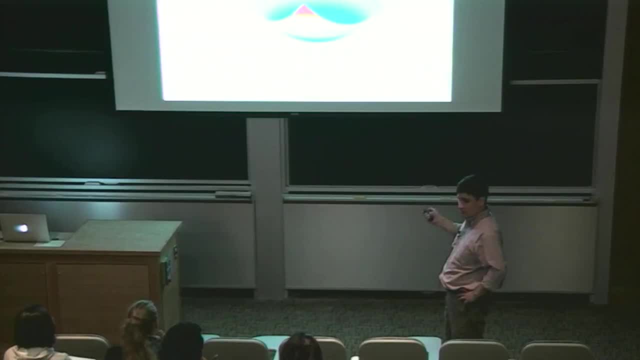 live inside this little blue circle. It could be d. It could be that x1 and x2 live on the surface of this circle, right on the circumference of this circle. That could be the constraint. Okay, So these are the sorts of problems we want to solve. d is called the feasible set. 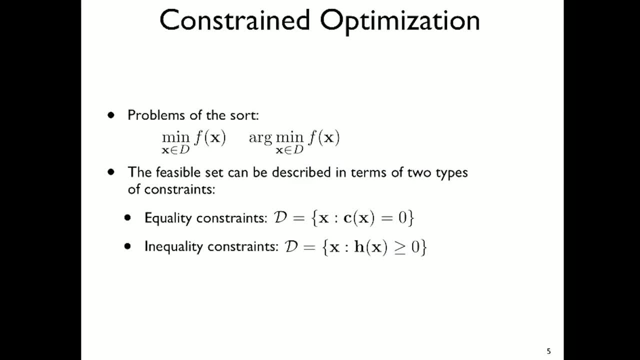 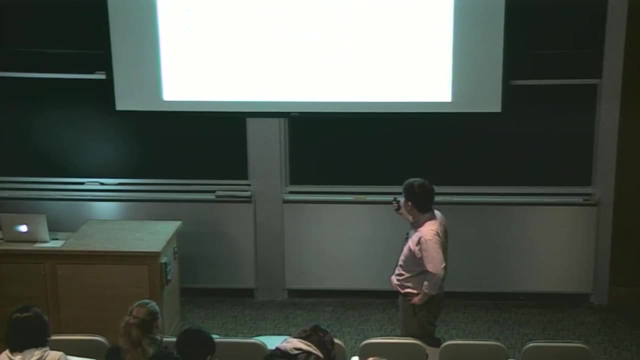 right, It can be described in terms of really two types of constraints. One is what we call equality constraints. So d can be the set of values x, such that some nominal nonlinear function c of x is equal to 0.. Okay, So it's the set of points that satisfy this. 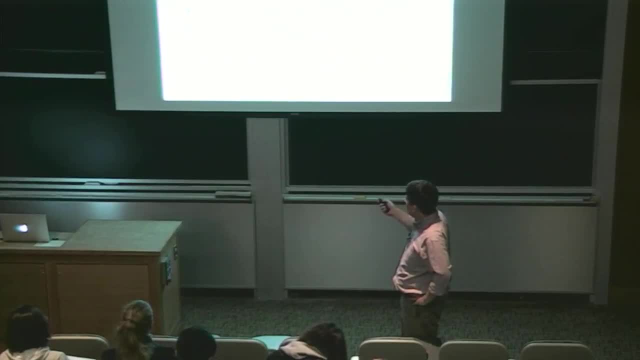 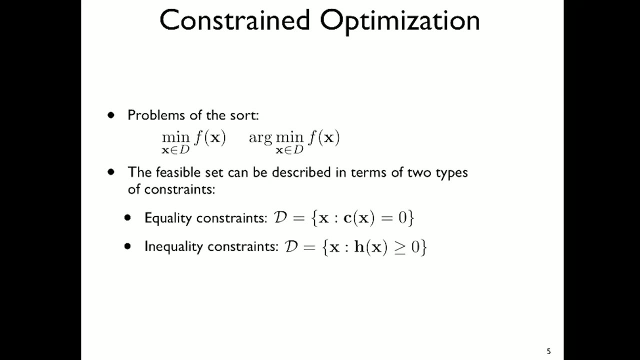 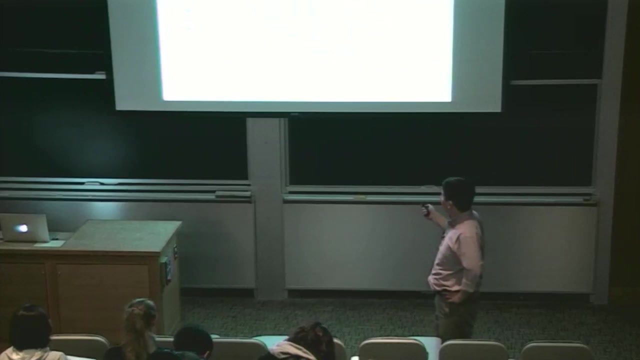 nonlinear equation And among those points we want to know which one produces the minimum in the objective function. Or it could be an inequality constraint. So d could be the set of points such that some nonlinear function h of x is by convention positive. Okay, 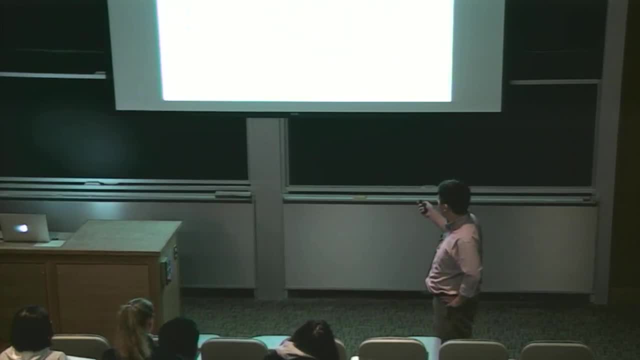 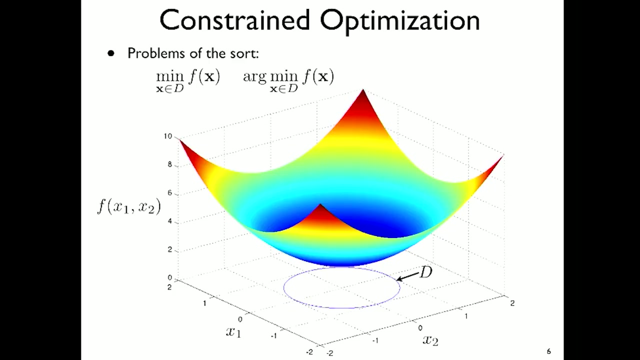 So h of x could represent, for example, the interior of a circle And c of x could represent the circumference of a circle, Right, And we would have nonlinear equations that reflect those values of x that satisfy those sorts of geometries. Okay So equality, constraint, right points that lie on this. 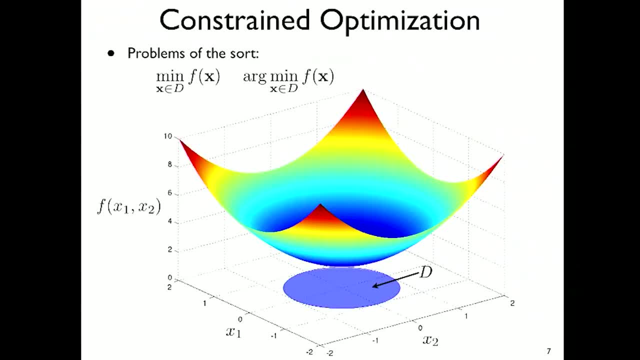 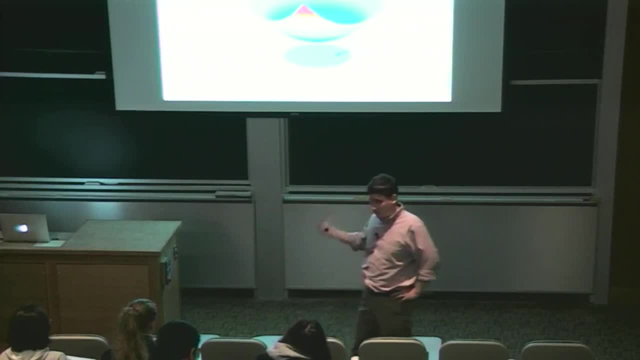 circle, Inequality, constraint points that lie within this circle. The shape of the feasible set is constrained by the problem that you're actually interested in, right? So it's easy for me to draw circles in the plane, because that's a shape you're familiar with. But 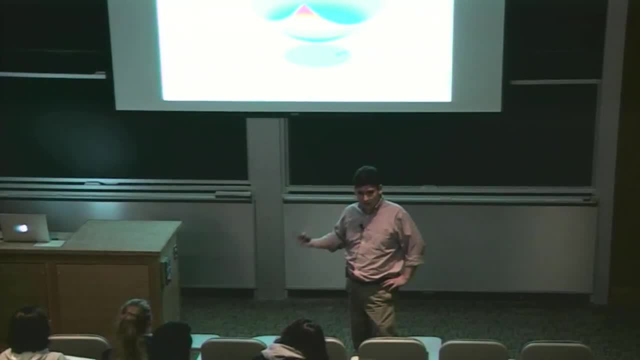 actually it'll come from some sort of physical constraint on the engineering problem you're looking at, Like mole fractions need to be bigger than 0 and smaller than 1. And temperatures and absolute value have to be bigger than 0 and smaller than some value, because that's. 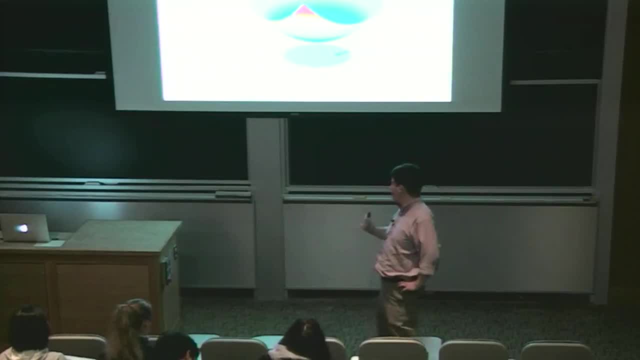 a safety factor on the process, Right? So these set up the constraints on various sorts of optimization problems that we're interested in. It could also be true that we're interested in, say, optimization in the domain outside of this circle too, Right, It could be on. 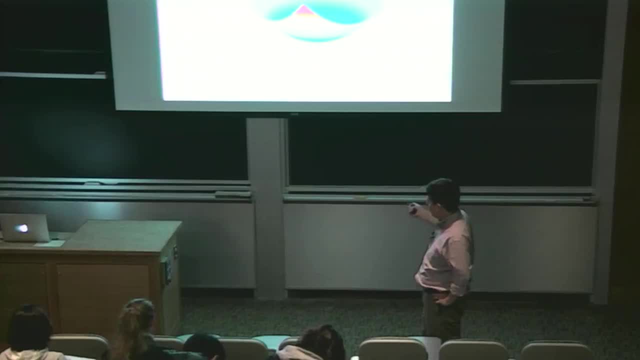 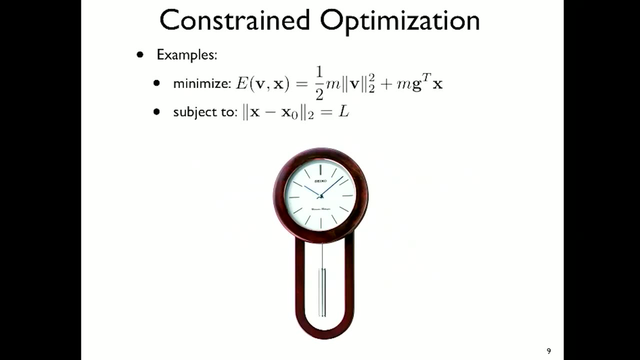 the inside, It could be on the outside Right. That's also an inequality constraint sort of problem. You know some of these already. Okay, They're familiar to you. So here's a classic one from mechanics: Right. Here's the total energy in a system for, say, a pendulum, Right. So 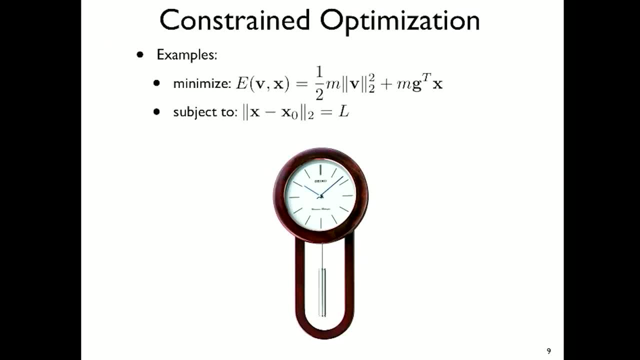 x is like the position of the tip of this pendulum and v is the velocity that it moves with. This is the kinetic energy, This is the potential energy, And we know the pendulum will come to rest in a place where the energy is minimized Right. 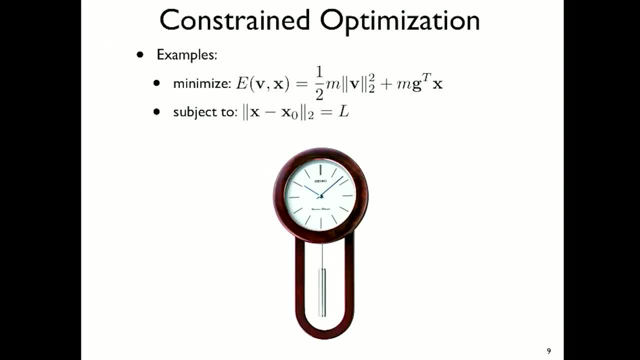 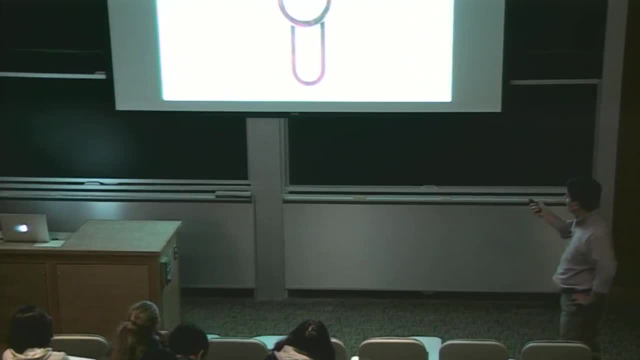 Well, the energy can only be minimized when the velocity here is 0, because any non-zero velocity will always push the energy content up. So it comes to rest, Right, It doesn't move, Right. And then there's some value of x at which the energy is minimized, Right. 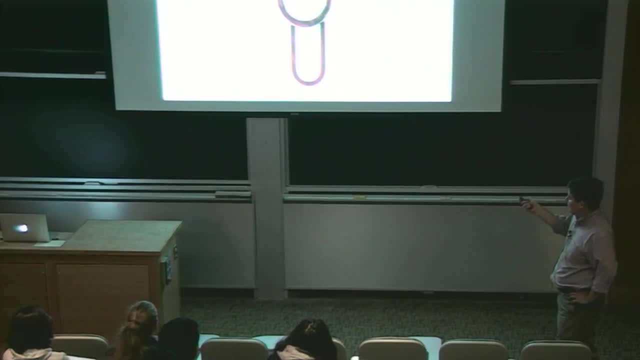 If there is no constraint that says that the pendulum is attached to some central axis, then I can always make the energy smaller by making x more and more negative. It just keeps falling. Right, There is no stopping point, But there's a constraint. Right, The 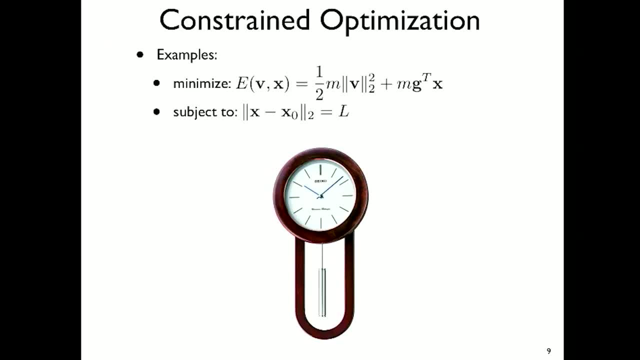 distance between the tip of the pendulum and this central point Right, Some fixed distance, l. So this is an equality constraint sort of problem And we have to choose from the set of v and x the values subject to this constraint that minimize the total energy. 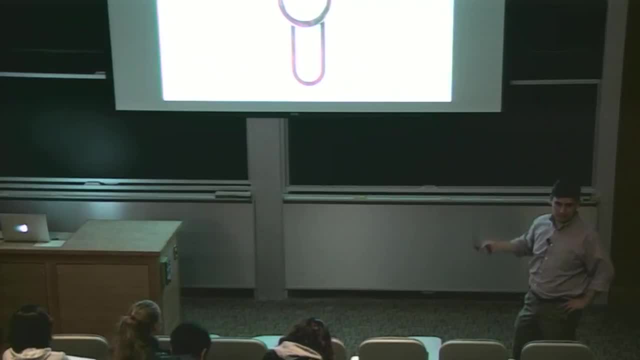 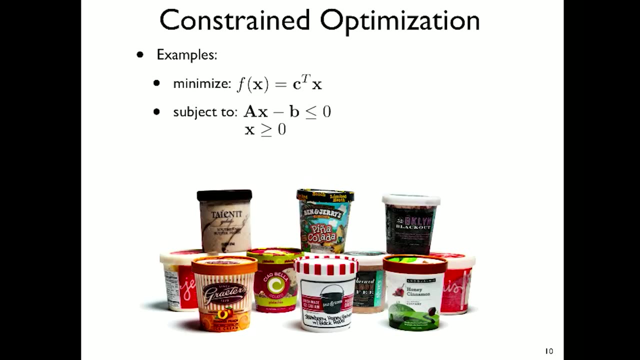 And that's this configuration of the pendulum here. So you know these sorts of problems already. But we talked about this one Right Linear sorts of programs. These are optimization problems where the objective function is linear Right And then there's a constraint, that 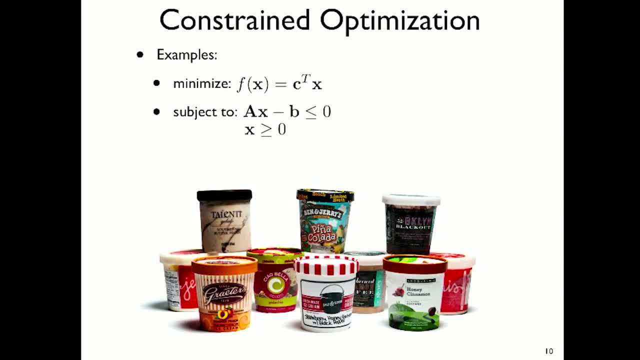 is linear in the design variables, Right? So it's just the dot product between x and some vector c that weights the different design options against each other. OK, So we talked about ice cream. Yes, this is all premium ice cream because it comes in the small containers. 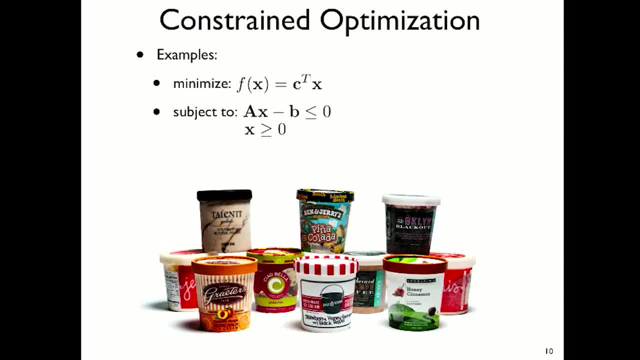 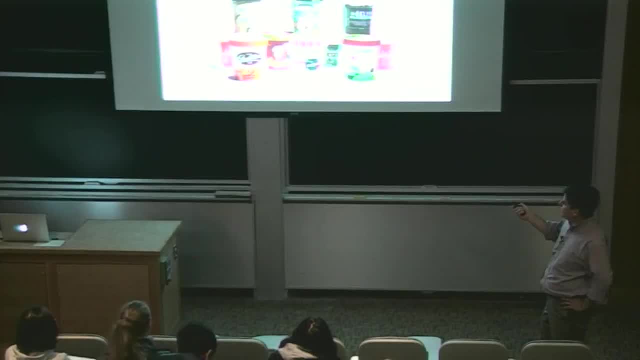 Right Subject to different constraints. So those constraints can be things like: oh x has to be positive, because we can't make negative amounts of ice cream, And maybe we've done market research that tells us that the market can only tolerate certain ratios of different. 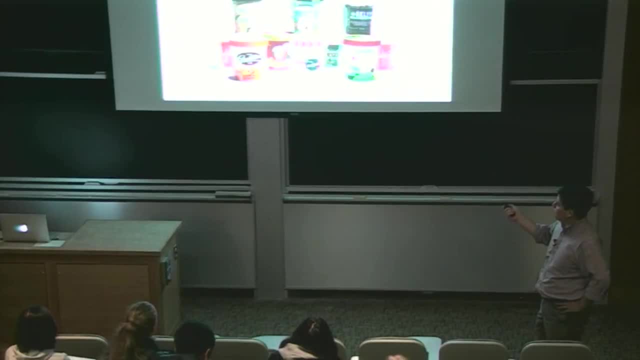 types of ice cream And that may be some set of linear equations that describe that market research, that sort of bound, the upper values of how much ice cream we can put out on the market, And then we try to choose the optimal blend of, you know, pina colada and strawberry to sell. OK. 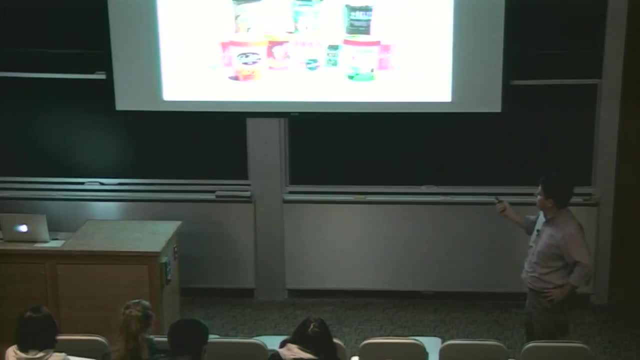 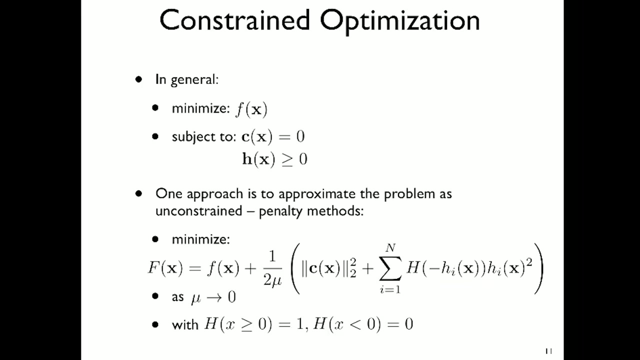 So those are linear programs. OK, This is an- I mean, this is an- inequality constrained optimization. OK, In general we might write these problems like this. We might say: minimize f of x subject to the constraint that c of x is 0 and h of x is positive. Right, So minimize it over the values of x that satisfy these. 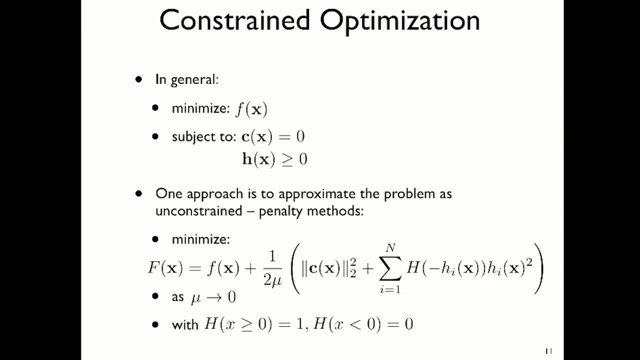 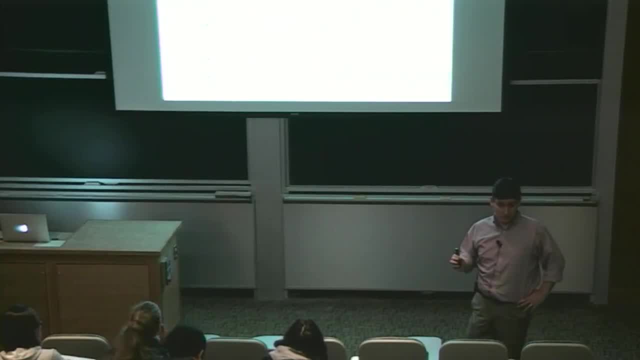 two constraints, And there's an old approach discussed in the literature and it's not used. I'm going to describe it to you and then I want you to try to figure out why it's not used. OK, And it's called the penalty method, And the penalty method works this way. It. 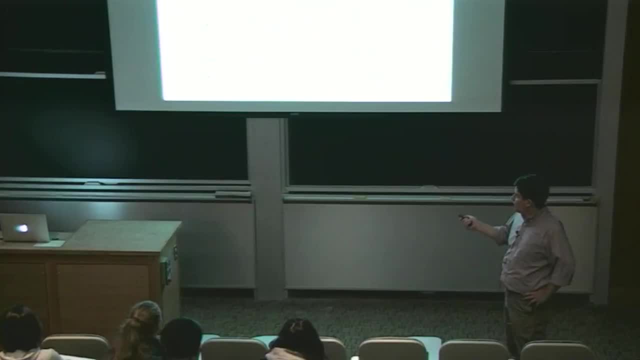 says, define a new objective function which is our old objective function, And then we're going to define a new objective function plus some penalty for violating the constraints. How does that penalty work? So we know that we want values of x for which c of x is equal. 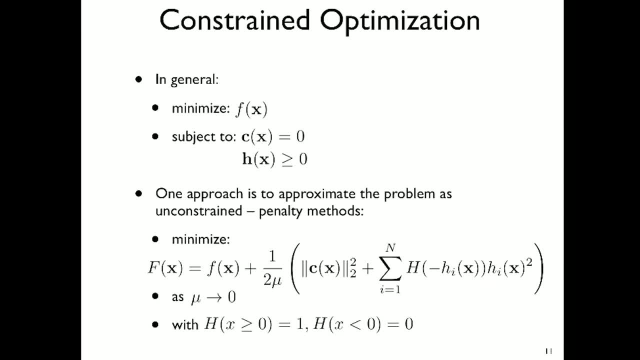 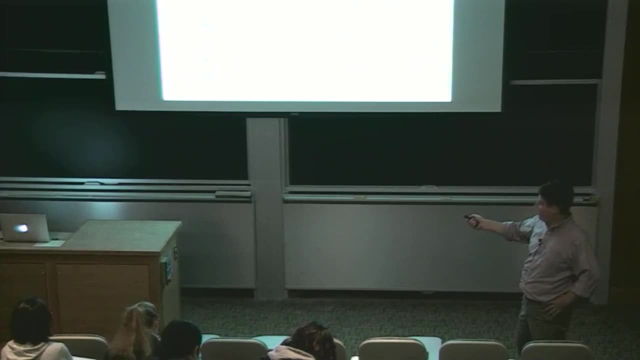 to 0.. OK, So if we add to our objective function the norm of c of x, this is a positive quantity. OK, This is a positive quantity. Whenever x doesn't satisfy the constraint, this positive quantity will be, will give us a bigger value for this objective function. f Right Then. 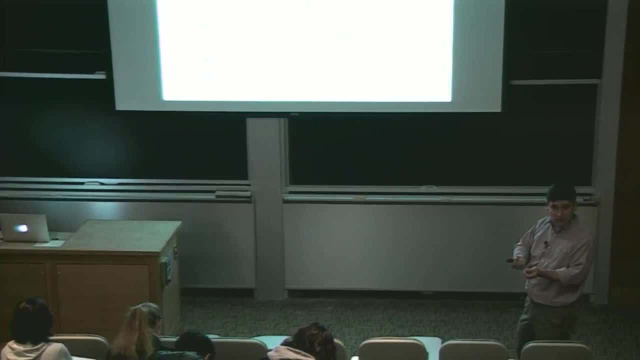 if c of x was 0. Right, So we're going to define a new objective function which is a positive function which is equal to 0. So we penalize right points which don't satisfy the constraint, And in the limit that this penalty factor mu here goes to 0, the penalties get large. 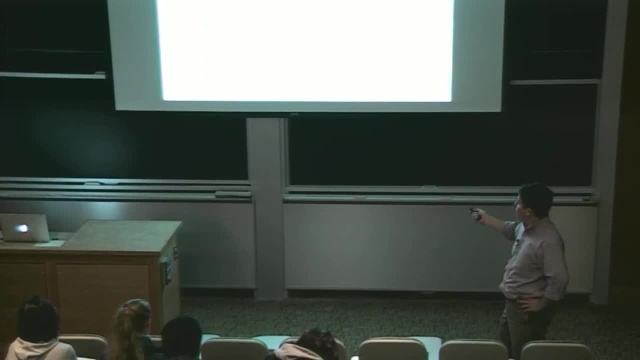 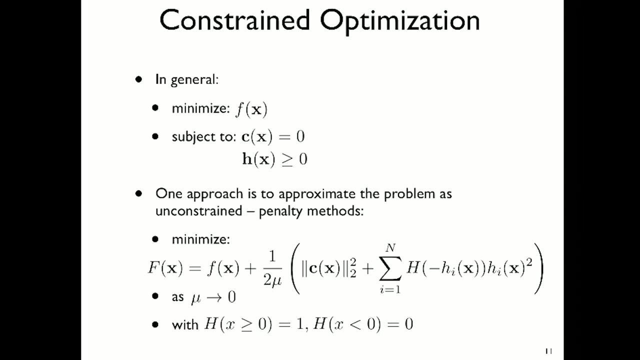 OK, So large that our solution will have to prefer right satisfying the constraints. There's another penalty factor over here which is identical to this one, but for the inequality constraint It says. it says: take a heavy side step. function Right For which is equal to one Right When the value of its argument is positive. 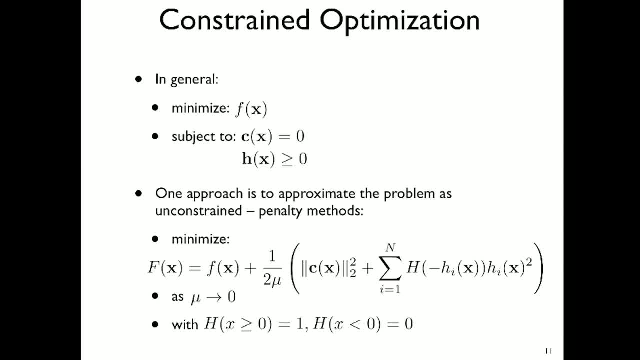 and it's equal to zero when the value of its argument is negative Right. So whenever I violate my each of my inequality constraints, h, i of X, Right, Turn on this heavy side step function, make it equal to one and then multiply it by the value of the constraint square. 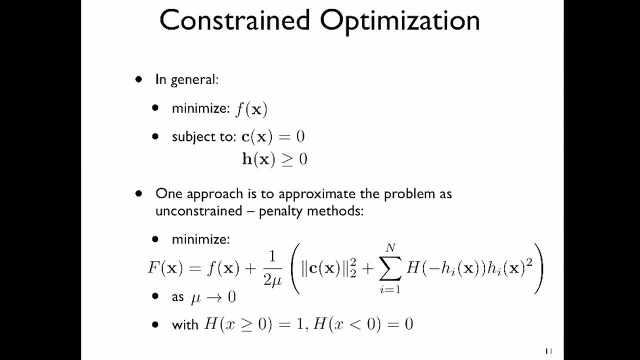 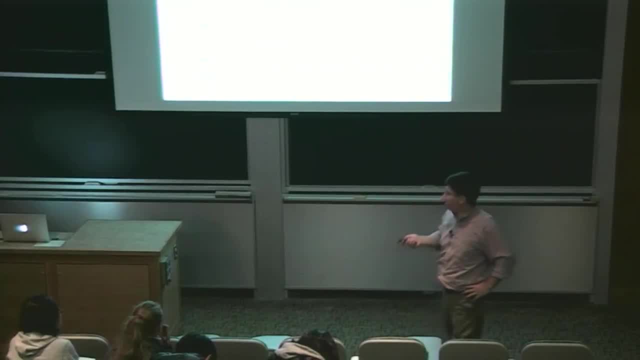 to a positive number, Right, So this is the inequality constraint penalty and this is the quality constraint penalty. People don't use this, though, So it makes sense. I take the limit that mu goes to 0. I'm going to have to prefer solutions that. 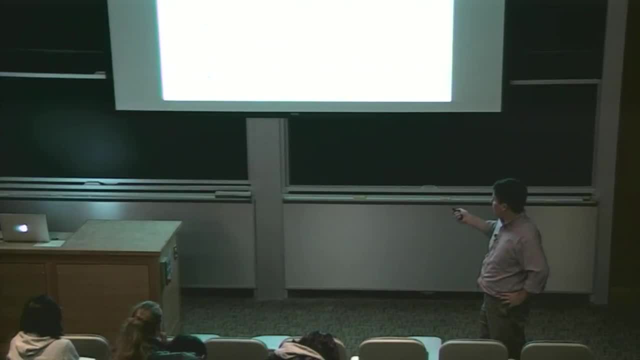 satisfy these constraints. Otherwise, if I don't satisfy these constraints, I can always move closer to a solution that satisfies the constraint And I'll bring down the value of the subjective function. I'll make it lower. So I'll always prefer these lower value solutions. 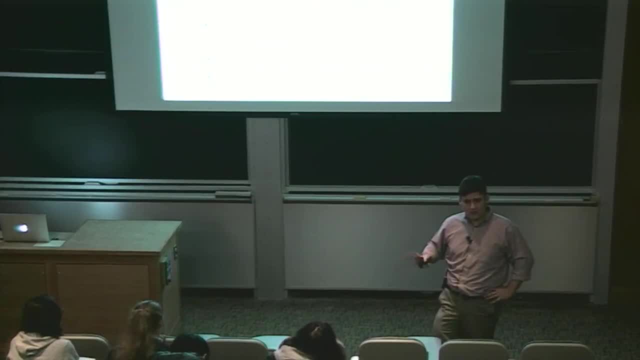 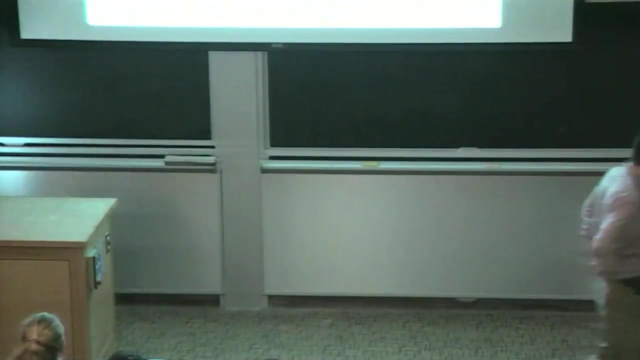 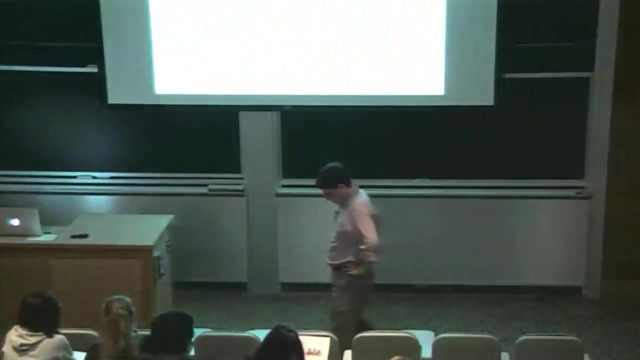 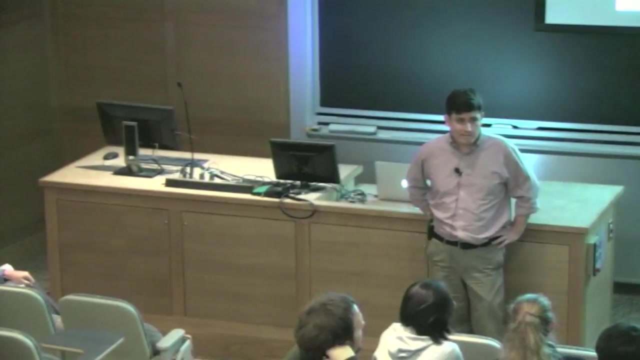 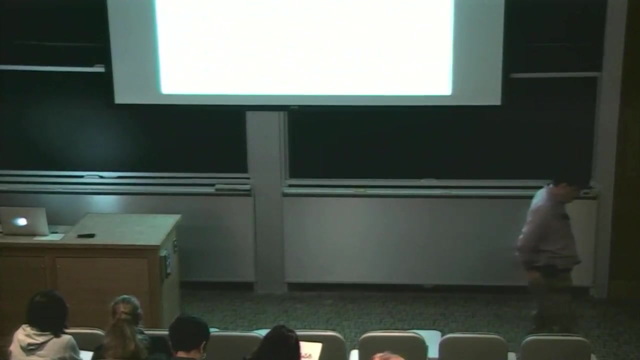 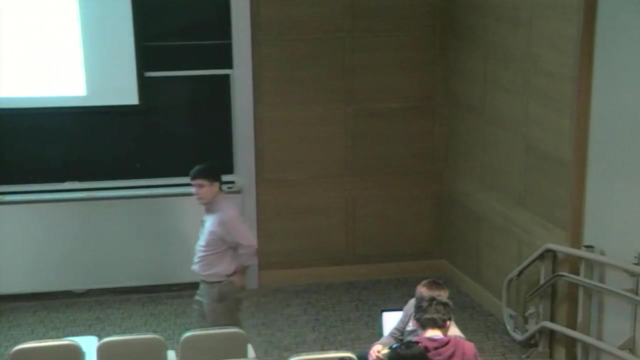 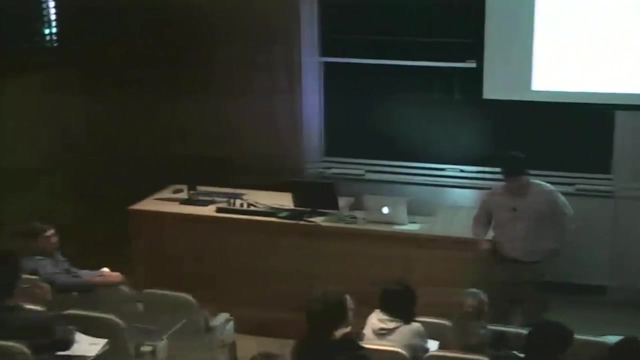 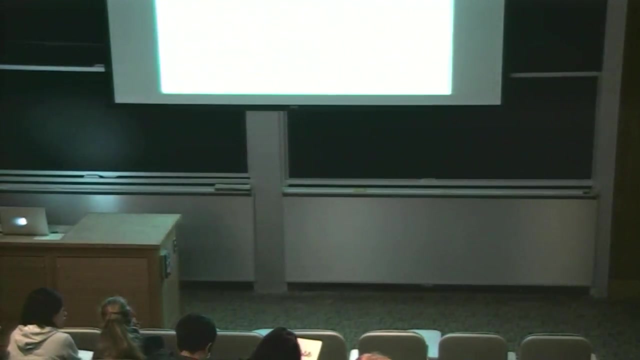 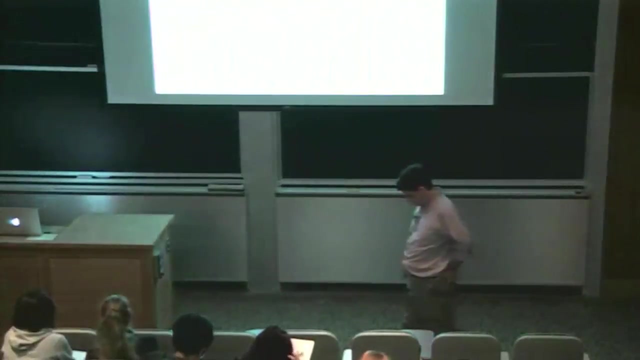 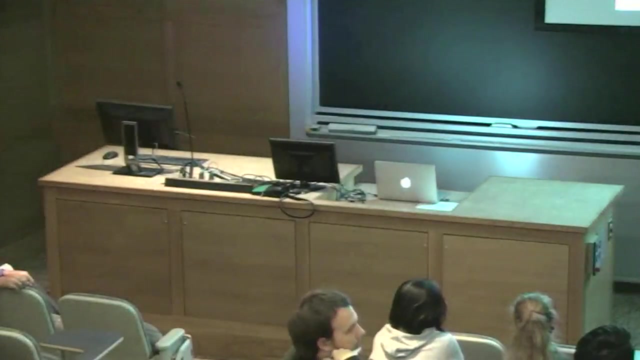 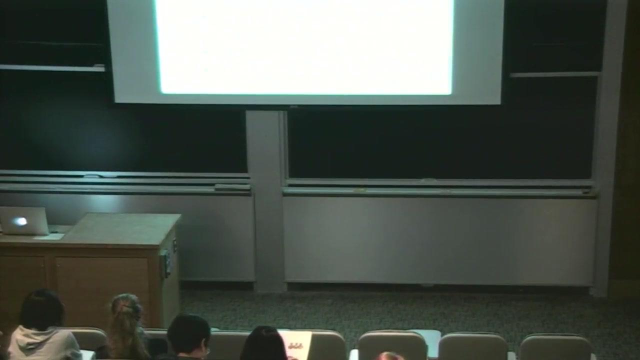 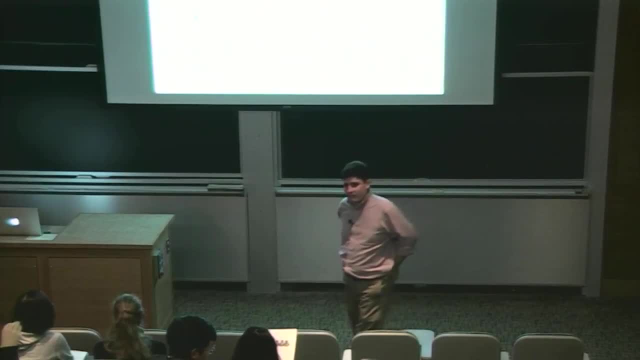 Why is this method a problem? I heard the volume go up at some point, which means either you switched topics and felt more comfortable talking about that than this, or maybe you guys were coming to some conclusions or had some ideas about why this might be a bad idea. 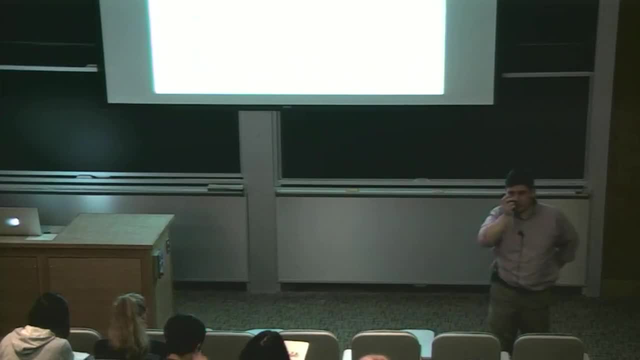 Do you want to volunteer some of what you were talking about? Yeah, Hirsch. Well, that's an interesting idea. So yeah, so if we have a non-convex optimization problem, there could be some issues with f of x. 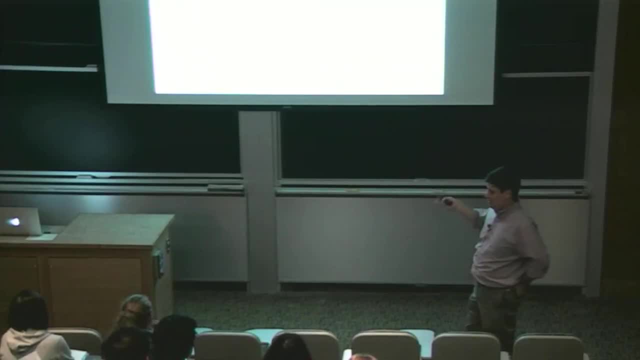 and maybe f of x runs away so fast that I can never make the penalty big enough to enforce the constraint. That's actually a really interesting idea and I like the idea of comparing the magnitude of these two terms. I think that's on the right track. 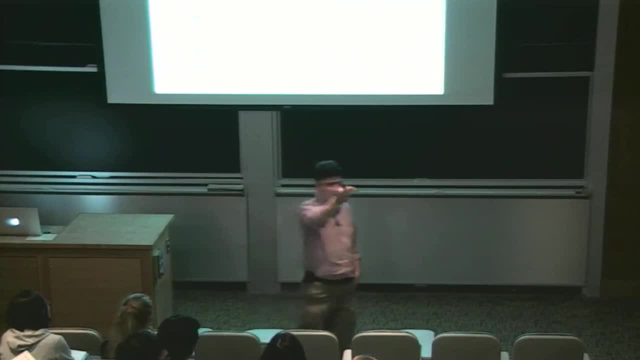 Were there some other ideas about why you might not do this? Different ideas- Yeah Well, you know that's an interesting idea, but actually the two terms in the parentheses here are both positive, right, So they're only going to be minimized. 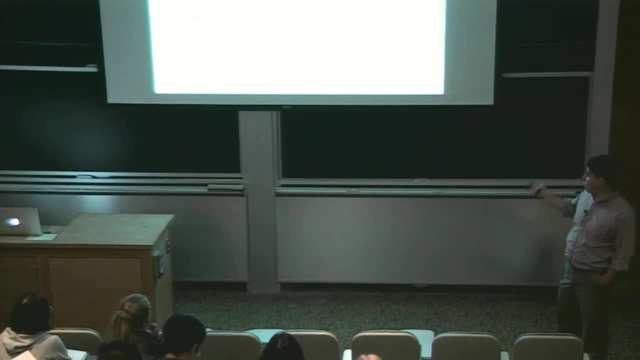 when I satisfy the constraints. So the local minimum of the terms in parentheses sit on or within the boundaries of the feasible set that we're looking at. So by construction actually, we're going to be able to satisfy them because the local minimum of these points 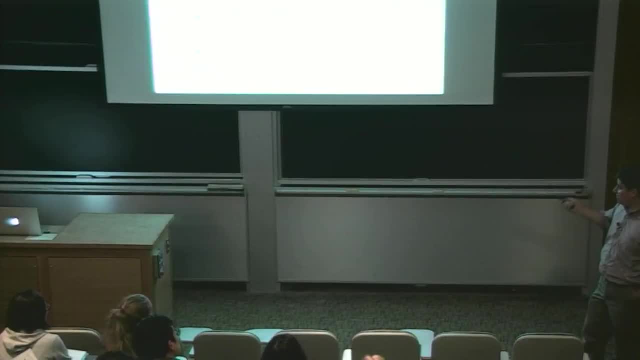 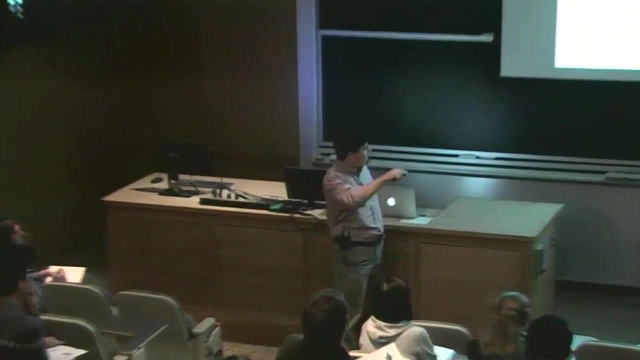 sits on these boundaries. These terms are minimized by satisfying the constraints. Other ideas: Yeah, What's that? Oh, this is a good point, right, The iterates. this is an unconstrained optimization problem. I'm just going to minimize. 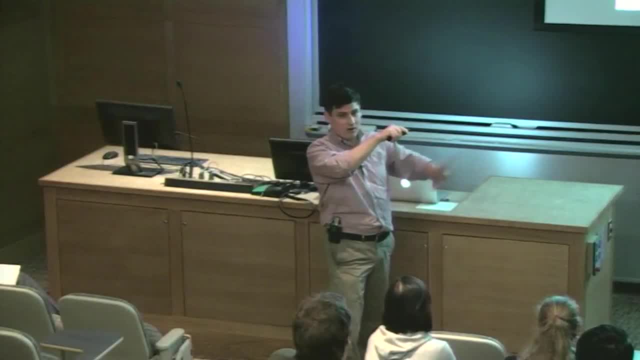 this objective function. it's like what Hirsch said: right, I can go anywhere I want in the domain. I'm going to minimize this objective function, then I'm going to try to take the limit as mu goes to zero. The iterates don't have to be feasible. 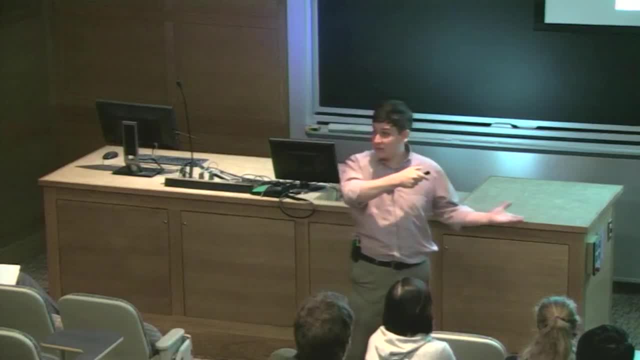 Maybe I can't even evaluate f of x if the iterates aren't feasible. That's an excellent point, right, That could be an issue Anything else? Were there some other ideas? Sure, I feel like, if your iterates are unfeasible, 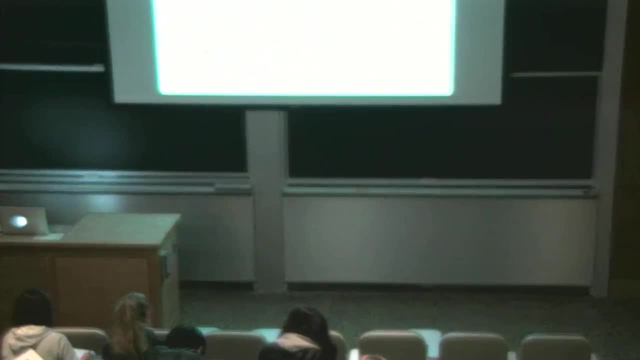 and you converge the domain boundary, you may have done your whole optimization and it isn't really feasible. You don't actually know what the objective does inside the region. I think that's a good point: The boundary from outside without knowing what it is. 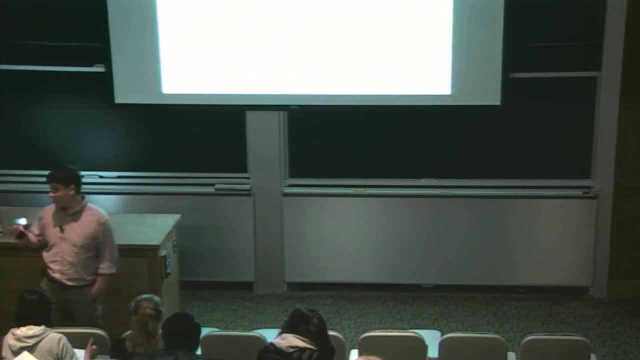 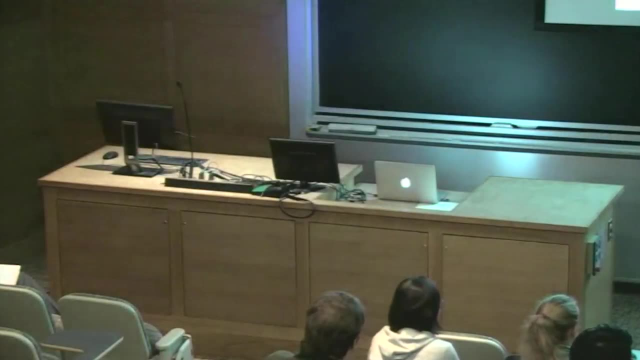 Sure. So you'll see. actually, the right way to do this is to use what's called interior point methods, which live inside the domain. This is an excellent point. There's another issue with this, that's. I think it's actually less subtle than some of these ideas. 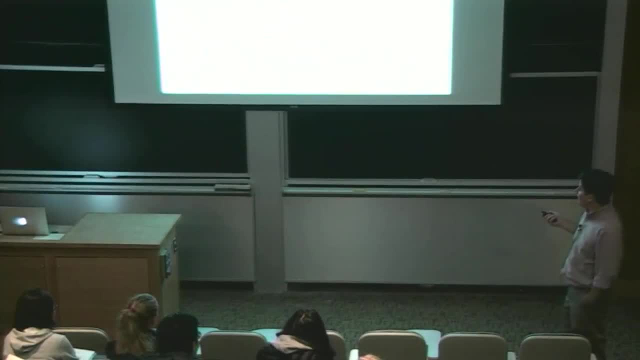 which are all. they're all correct. actually, These can be problems with this sort of penalty method. As I take the limit that mu goes to zero, the penalty function becomes large for all points outside the domain. They can become larger than f for those points. 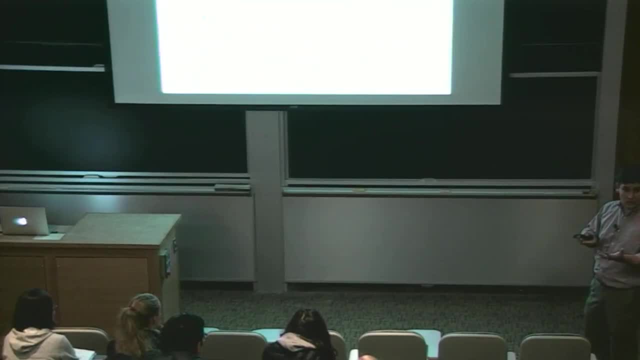 And so there's some practical issues about comparing these two terms against each other. I may not have sufficient accuracy, sufficient number of digits to accurately add these two terms together, So I may prefer to find some point that lives on the boundary of the domain. 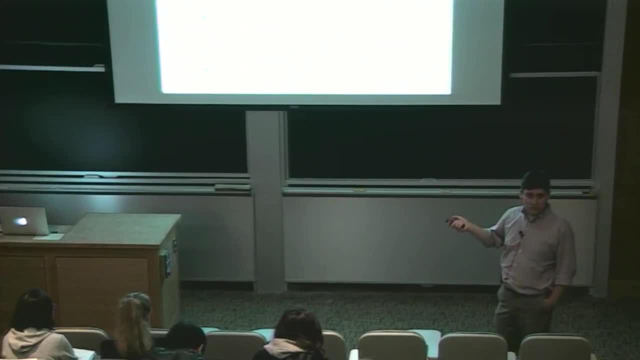 as mu goes to zero, but I can't guarantee that it was a minima of f on that domain or within that feasible set. So a lot of practical issues that suggest this is a bad idea. This is an old idea. People knew this was bad for a long time. 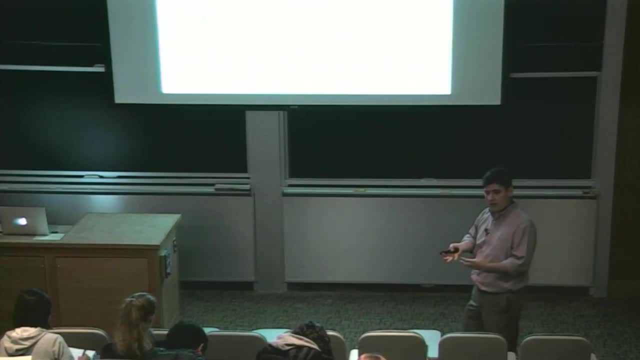 It seems natural, though It seems like a good way to transform from these constrained optimization problems to something we know how to solve an unconstrained optimization problem, But actually it turns out not to be such a great way to do it, Okay. 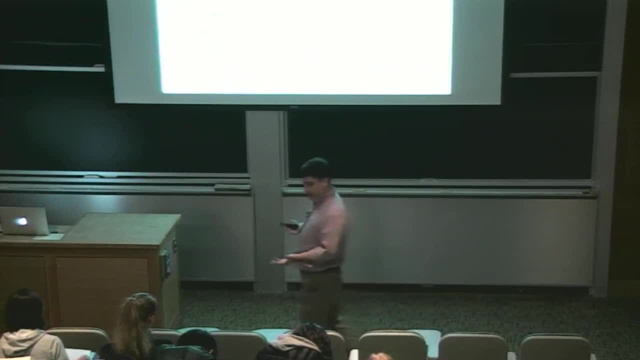 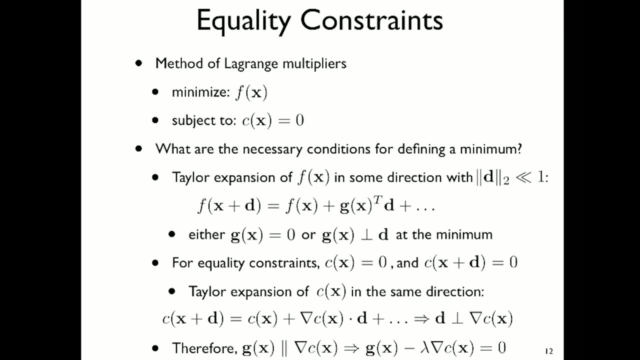 So let's talk about separating out these two different methods from each other, or these two different problems. Let's talk first about equality constraints and then we'll talk about inequality constraints. So, equality constrained optimization problems look like this: right: Minimize f of x subject to c of x equals zero. 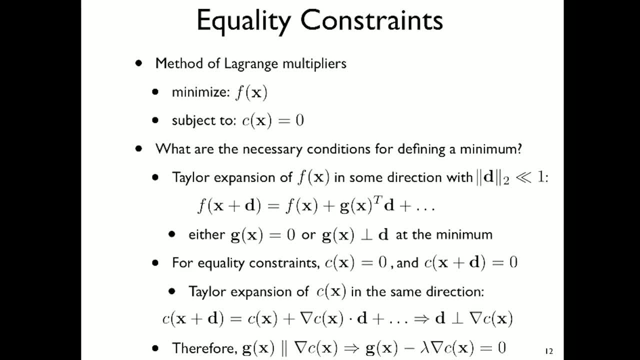 and let's make it even easier. Rather than having some vector of equality constraints, let's just have a single equation that we have to satisfy for that equality constraint, like the equation for a circle, right Solutions have to sit on the circumference of 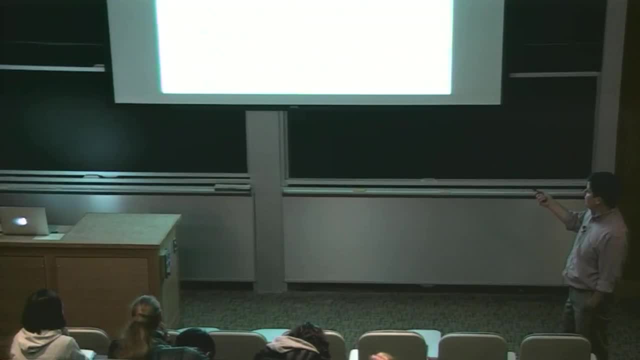 right Of a circle. okay, So one equation that we have to satisfy. You might ask again: what are the necessary conditions for defining a minimum? Okay, That's what we used when we had equality or when we had unconstrained optimization. 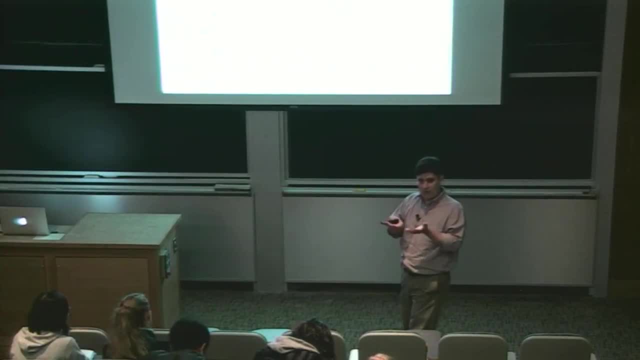 First, we had to define what a minimum was right, And we found that minima were critical points, places where the gradient of the objective function was zero. Okay, That doesn't have to be true anymore. right Now, the minima has to live on this boundary right. 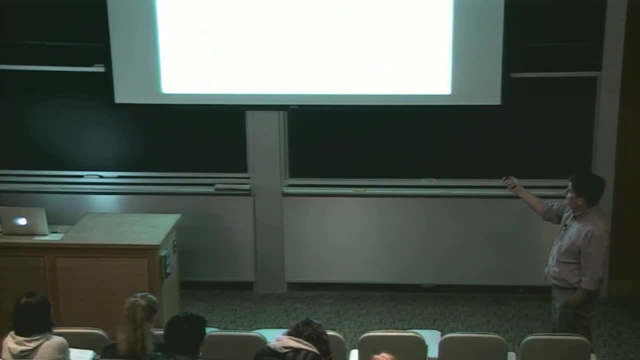 of some domain It has to live in this set of points. c of x equals zero and the gradient of f is not necessarily zero at that minimal point. okay, But you might guess right that Taylor expansions are the way to figure out, okay. 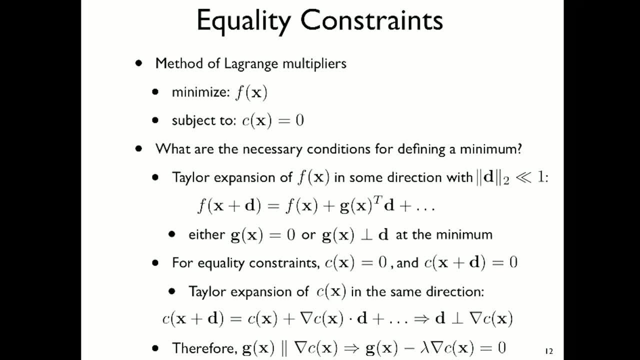 Taylor expansions are the way to figure out, the way to figure out what the appropriate conditions for a minima are. So let's take f of x and let's expand it, do a Taylor expansion in some direction. d okay, So we'll take a step away from it. 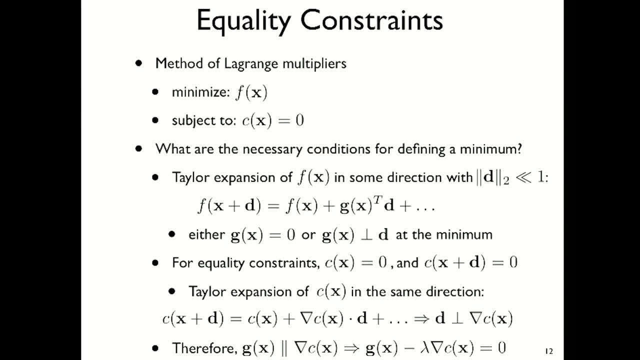 and we'll take a step away from it. and we'll take a step away from it and we'll take a step away from x, which is small right in some direction, d, So f of x plus d is f of x plus g, dot d right. 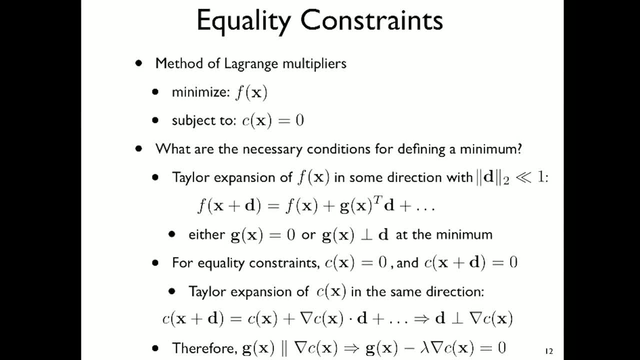 the dot product between the gradient of f and d And at a minimum right, either the gradient is zero or the gradient is perpendicular to this direction. we moved in d. okay, We know that, because this term right this term. 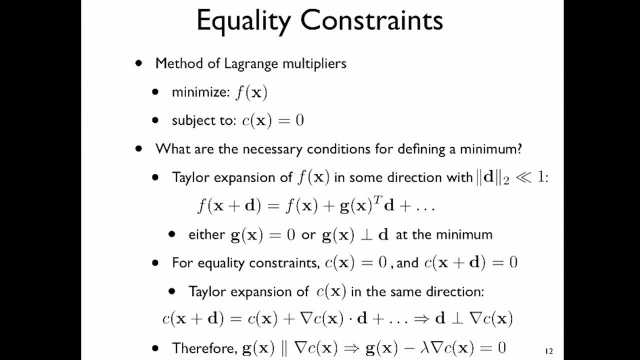 is going to increase will change the value of f of x. It'll either make it bigger or smaller, depending on whether it's positive or negative. In either case, it'll say that this point x can't be a minimum right. 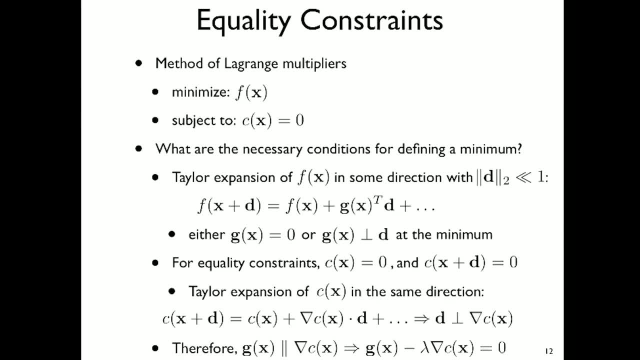 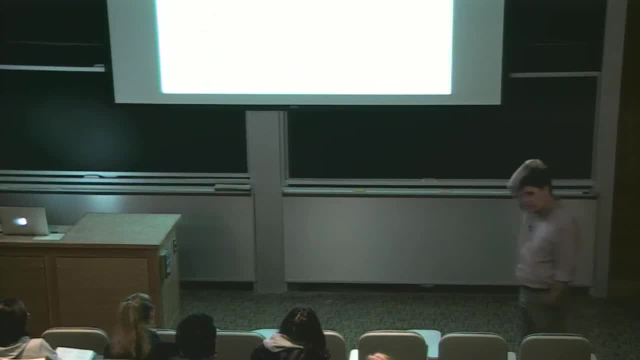 unless this term is exactly equal to zero in the limit that d becomes small. So either the gradient is zero or the gradient is orthogonal to this direction d. we stepped in And d was arbitrary, right? We just said: take a step in a direction d. okay, 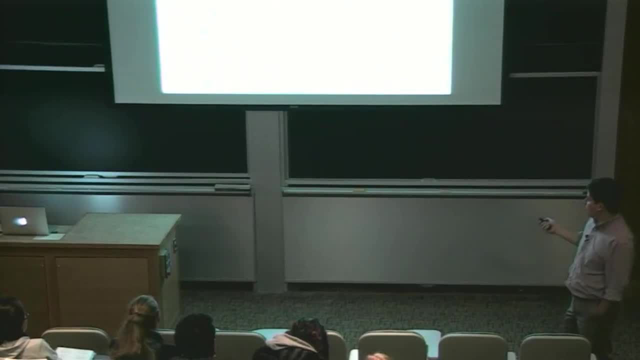 Let's take our equality constraint and do the same sort of Taylor expansion. okay, Because we know, right, if we're searching for a minima along this curve, c of x better be equal to zero, It better satisfy the constraint. And also c of x plus d, right? 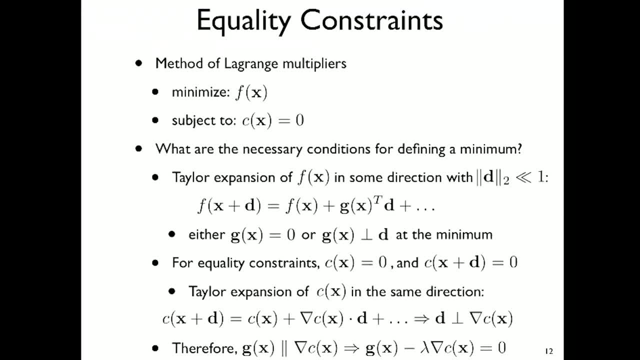 that little step in the direction. d should also satisfy the constraint, right? We want to study only the feasible set of values, okay, So actually d wasn't arbitrary. d had to satisfy this constraint And when I took this little step right. 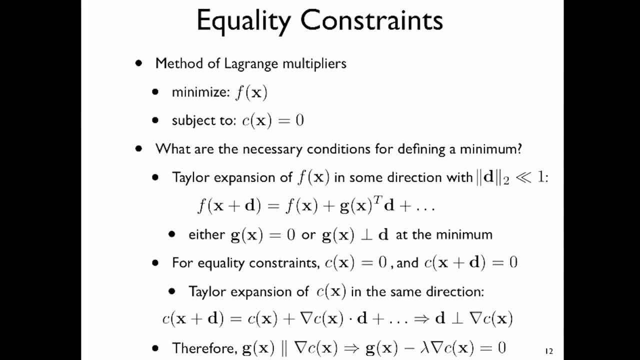 d had to satisfy this constraint. And when I took this little step right, d had to satisfy this constraint. And when I took this little step right c of x plus d had to be equal to zero. So again, we'll take now a Taylor expansion. 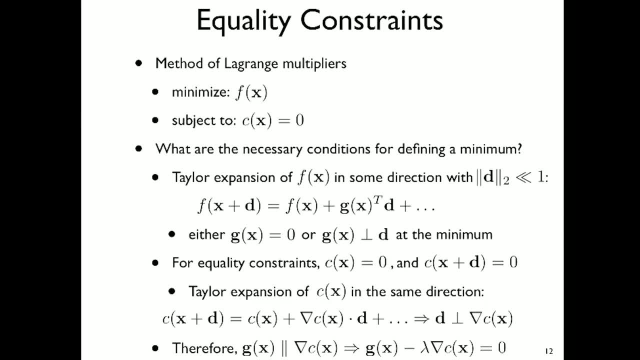 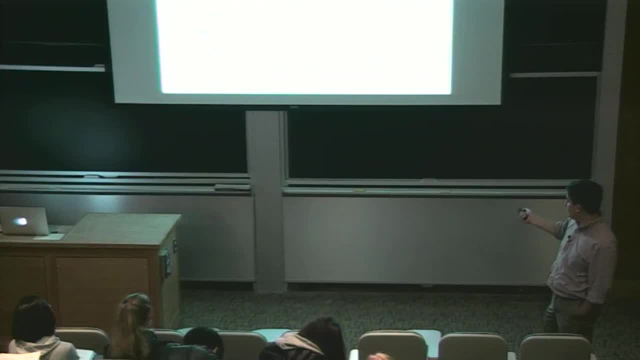 of c of x plus d, which is c of x plus grad of c of x dotted with d. okay, And that implies, right, that d must be perpendicular to the gradient of c of x. okay, Because c of x plus d has to be zero. 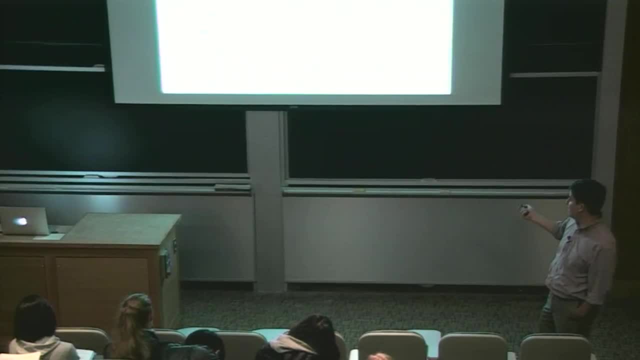 and c of x has to be zero. So the gradient of c of x dot d to leading order right has also got to be equal to zero. So d and the gradient in c are perpendicular And d and the gradient in g have to be perpendicular. 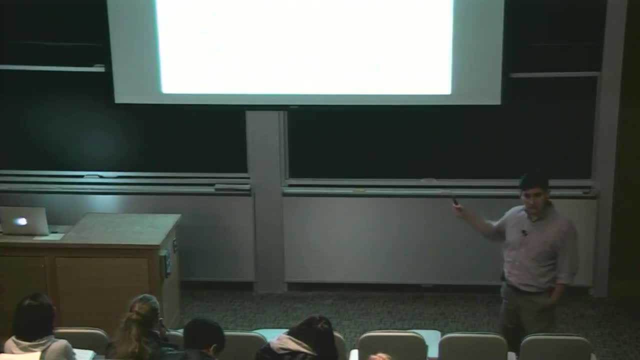 at a minimum. okay, That's going to define the minimum. on this equality constraint set. Does that make sense, right? c satisfies the constraint. c plus d satisfies the constraint. If this is true, d has to be perpendicular to the gradient of c. 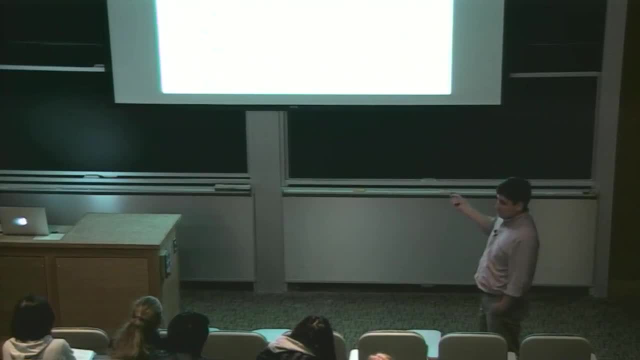 g has to be perpendicular to the gradient of d. d is in some sense arbitrary. still, okay, d has to satisfy a condition: that it's perpendicular to the gradient of c. but who knows right? There could be lots of vectors. 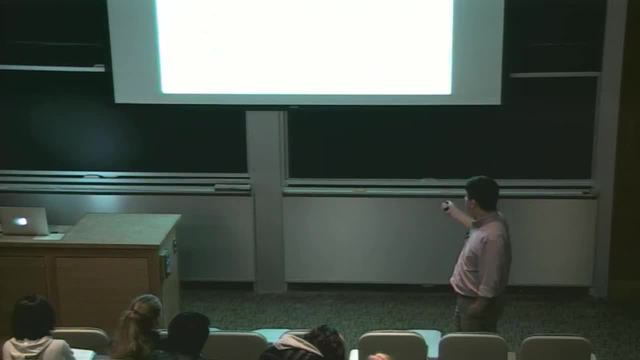 that are perpendicular to the gradient of c. So the only generic relationship between these two we can formulate is: g must be parallel to the gradient of c. right g is perpendicular to d. Gradient of c is perpendicular to d In the most generic way. 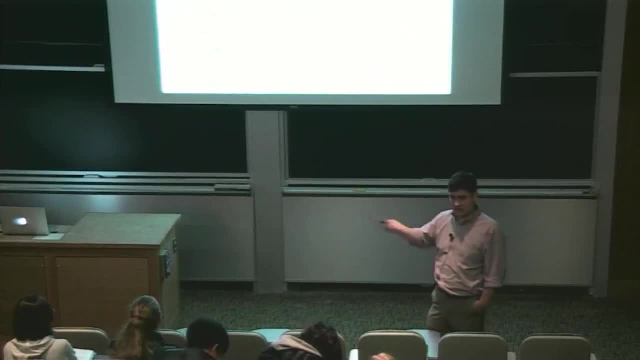 g and gradient of c should be parallel to each other. because d I can select arbitrarily from all the vectors in of the same dimension as x. okay, If g is parallel to the gradient of c, then I can write that g minus right. 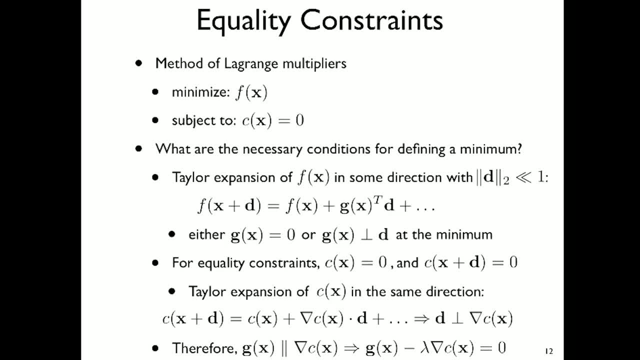 some scalar multiplied by the gradient of c is equal to zero right. That's an equivalent statement that g is parallel to the gradient of c. So that's a condition associated with points x that solve this equality constrained problem. The other condition is that point x 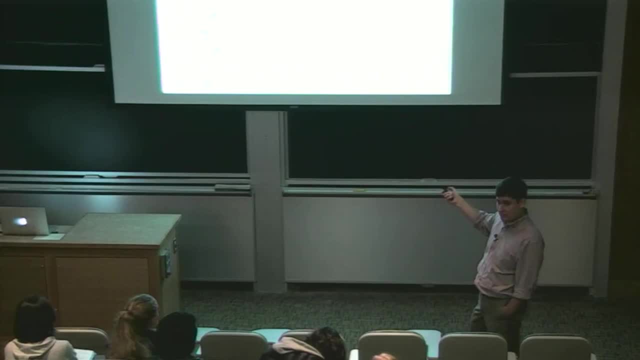 still has to satisfy the constraint. It still has to satisfy the equality constraint, right? But I introduced a new unknown- this lambda, okay- which is called the Lagrange multiplier. okay. So now I have one extra unknown, okay. but I have one extra equation. 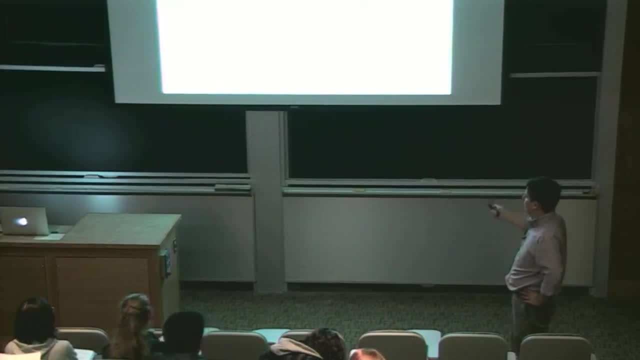 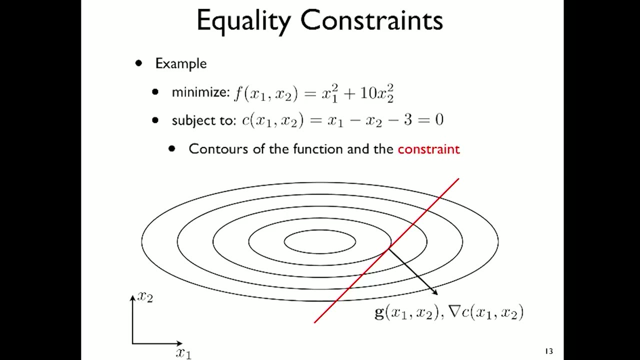 Let me give you a graphical depiction of this, and then I'll write down the formal equations again. So let's suppose we want to minimize, right, this parabolic function, subject to the constraint that the solution is going to be. So let's suppose that the solution is going to be. 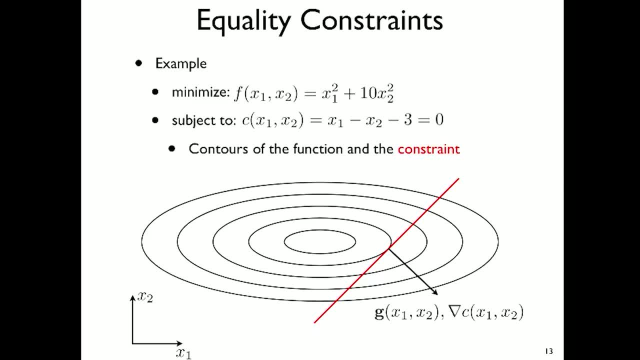 that the solution lives on the line. okay, So here's the contours of the function and the solution has to live on this line. okay, So I get to stand on this line and I get to walk and walk, and walk until I can't walk downhill anymore. 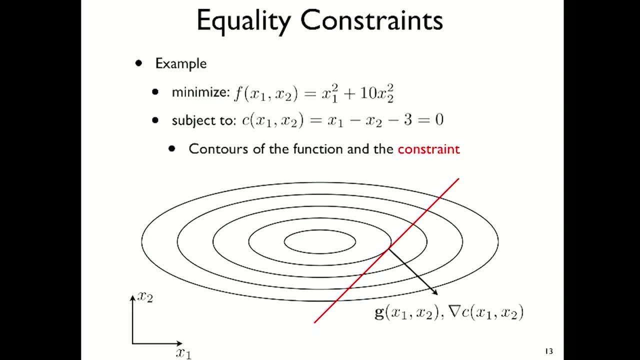 and I got to turn and walk uphill again, And you can see the point right. where I can't walk downhill anymore is the place where this constraint is parallel to the contour, or where I can't walk downhill anymore, Or where the gradient right 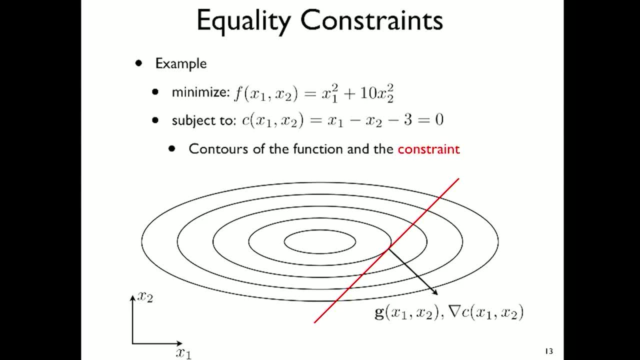 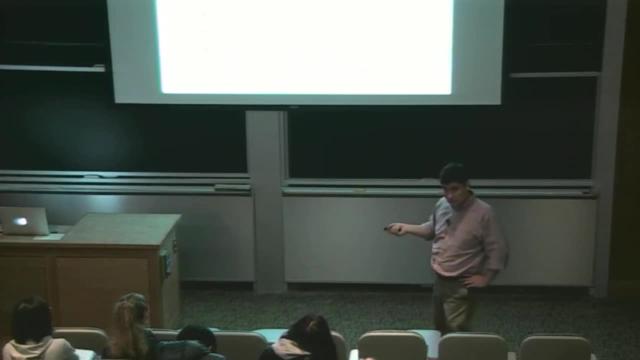 of the objective function is parallel to the gradient of the constraint. okay, So you can actually find this point by imagining yourself moving along this landscape. After I get to this point, I start going uphill again. right, So that's the method of Lagrange multipliers. 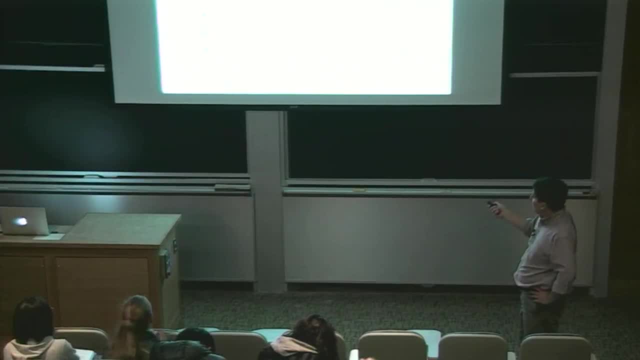 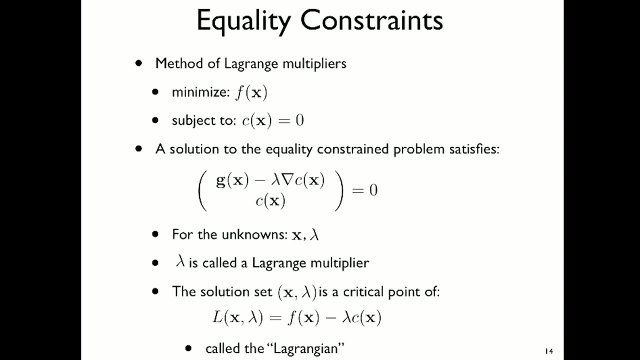 Minimize f of x, subject to this constraint, The solution is given by the point x, at which the gradient is parallel to the constraint- Okay, It's parallel to the gradient of c- and at which c is equal to zero, And you solve this system of nonlinear equations. 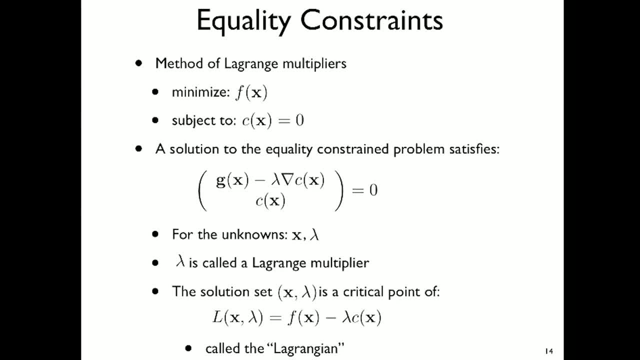 for two unknowns. One is x and the other is this unknown. lambda right, What is? you know how far stretched is the gradient relative in f relative to the gradient in c? So again, we've turned the minimization problem into a system of nonlinear equations. 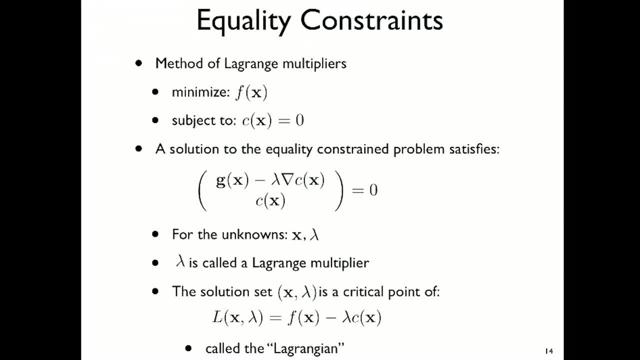 In order to satisfy the equality constraint, we've had to introduce another equation. This is the Lagrange multiplier. It turns out right. this solution set x and lambda is a critical point of something called the Lagrangian right. It's a function f of x minus lambda times c. okay. 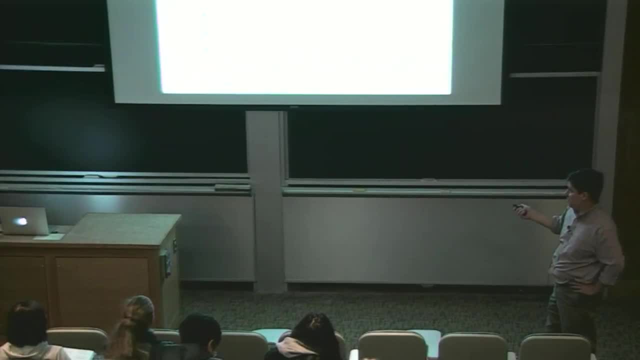 It's a critical point in x and lambda right of this nonlinear function called the Lagrangian. It's not a minimum of this function. unfortunately, It's a saddle point of the Lagrangian, it turns out Okay, So we're trying to find a saddle point of the Lagrangian. 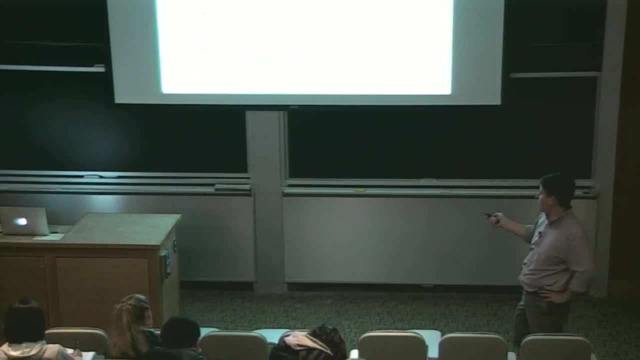 Does this make sense? Yes, Okay, We've got to be careful, of course. Just like with unconstrained optimization, we've actually got to check that our solution is a minimum right We can't take for granted. We can't suppose that our nonlinear solver 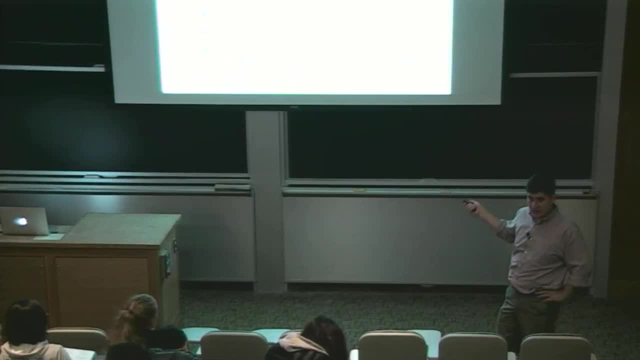 found a minimum when it solved this equation right. Other critical points can satisfy this equation too, So we've got to go back and try to check robustly whether it's a minimum or not, Or whether it's actually a minimum. But this is the method. 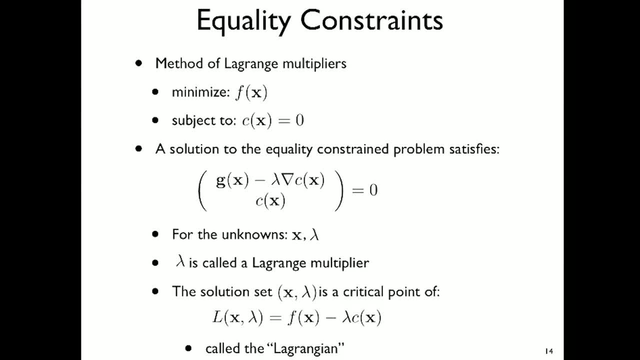 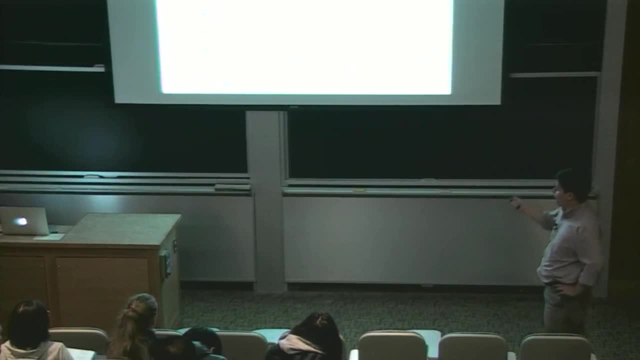 Introduce an additional unknown, the Lagrange multiplier, because you can show geometrically that the gradient of the objective function should be parallel to the gradient of the constraint at the minimum. Does that make sense? This picture make sense. Okay, So you know how to solve systems of nonlinear equations. 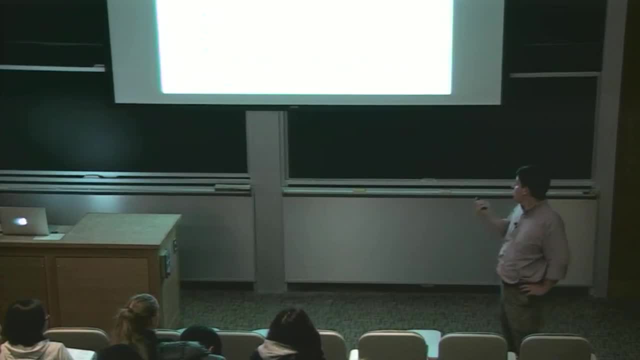 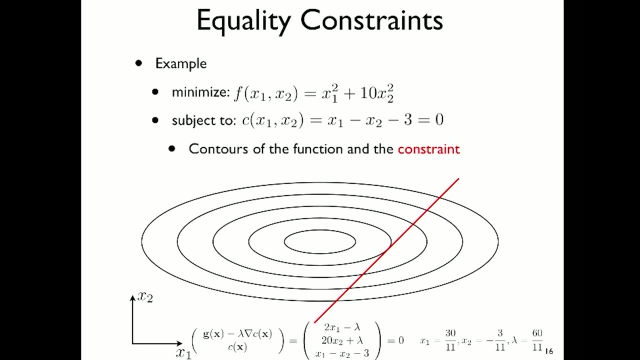 You know how to solve constrained optimization problems. Okay, So here's f, Here's c. right, We can actually write out what these equations are. right? So you can show that the gradient of x minus lambda, gradient of c, that's a vector 2x1 minus lambda and 20x2 plus lambda. 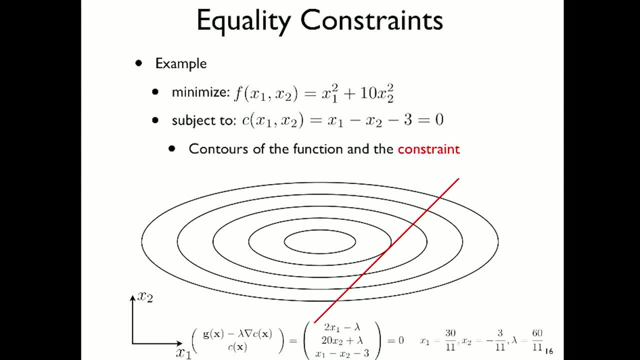 And c is the equation for this line down here. So x1 minus x2 minus 3.. And that's all got to be equal to 0, right? In this case? this is just a system of linear equations, So you can actually solve directly for x1,, x2,. 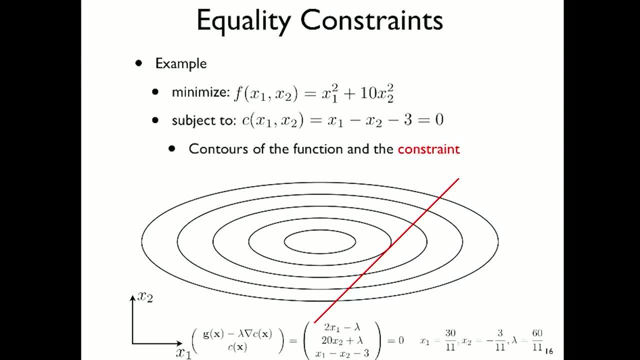 and lambda. okay, And it's not too difficult to find the solution for all three of these things by hand. okay, But in general right, these constraints can be nonlinear. The objective function doesn't have to be quadratic. Those are the easiest cases to look at. 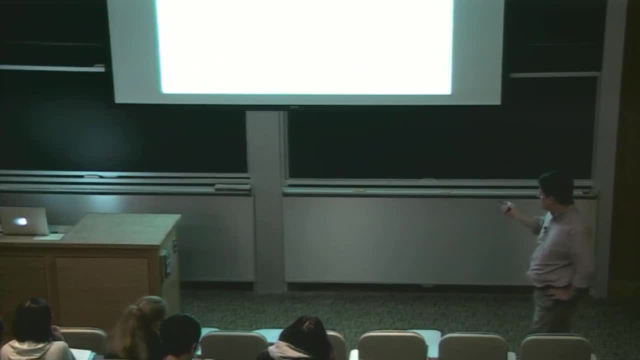 and the same methodology applies, okay. So you should check that you're able to do this right. This is the simplest possible equality constraint problem. You could do it by hand. You should check that you're actually able to do it, that you understand the steps that go into writing out these equations. 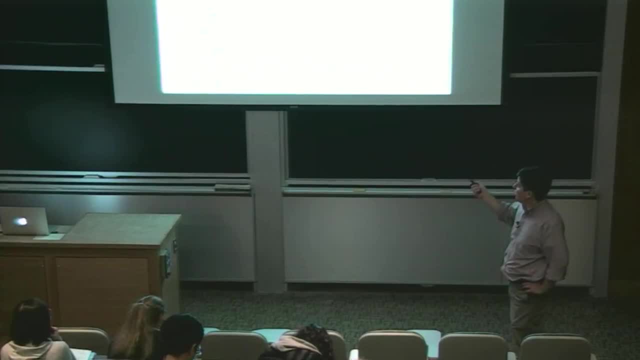 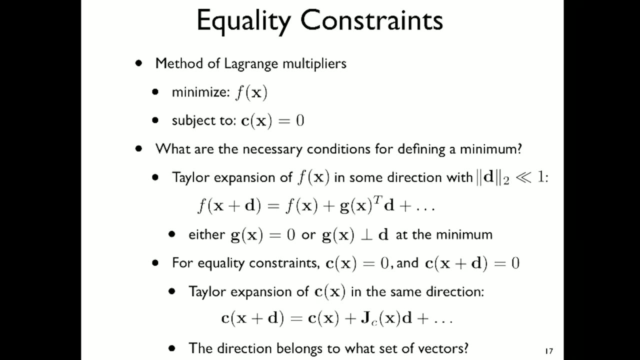 Okay, let's just take one step forward and look at a less generic case, one in which we have a vector-valued function that gives the equality constraints instead. So rather than one equation we have to satisfy, there may be many, okay. 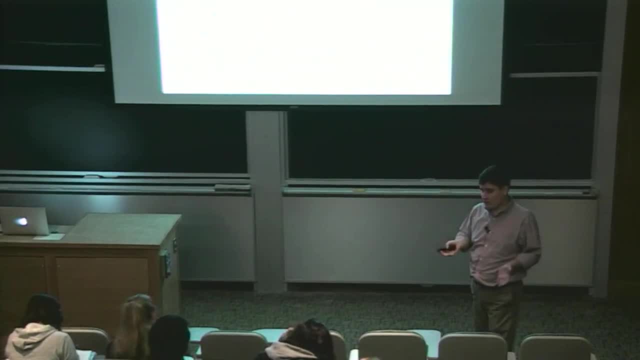 It's possible, right, that the feasible set doesn't have any solutions in it. right, It's possible that there is no x that satisfies all of these constraints simultaneously. That's a bad problem to have, right. You wouldn't like to have that problem very much. 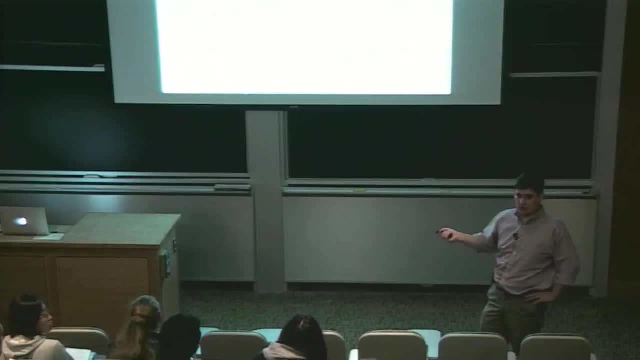 but it's possible that that's the case, But let's assume that there are solutions for the time being. okay, So there are x's that satisfy the equality constraint. Let's see if we can figure out again what the necessary conditions for defining a minima are. 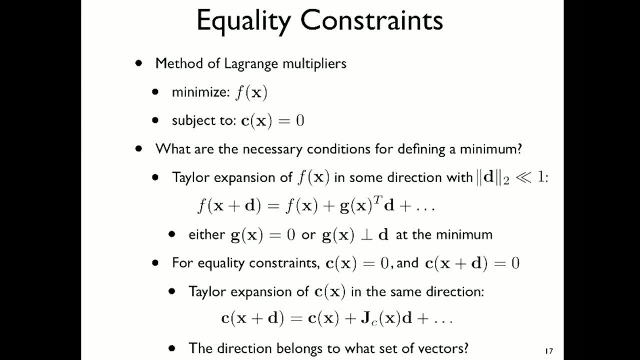 So same as before. let's Taylor expand f of x going in some direction d and let's make d a nice small step so we can just treat the f of x plus d as a linearized function. So we can see again that g has to be perpendicular. 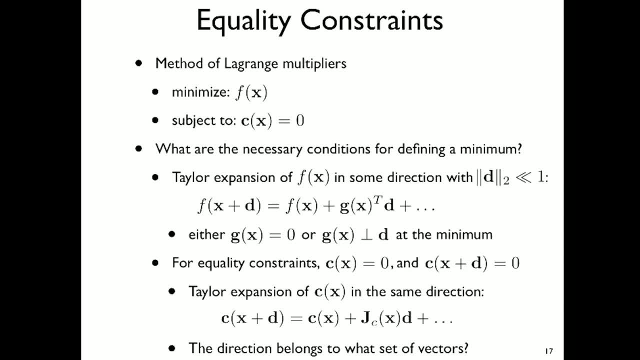 to this direction d if we're going to have a minima. Otherwise I could step in some direction d and I'll find either a smaller value of f of x plus d or a bigger value of f of x plus d. okay, So g has to be perpendicular to d. 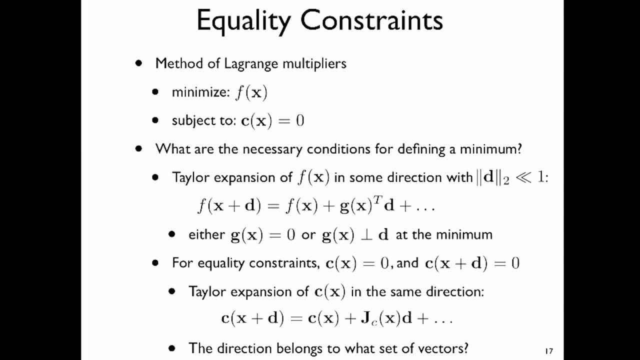 And for the equality constraints. again, they all have to satisfy, right, this equality constraint up there. So c of x has to be equal to zero, and c of x plus d also has to be equal to zero. And so right, if we take a Taylor expansion. 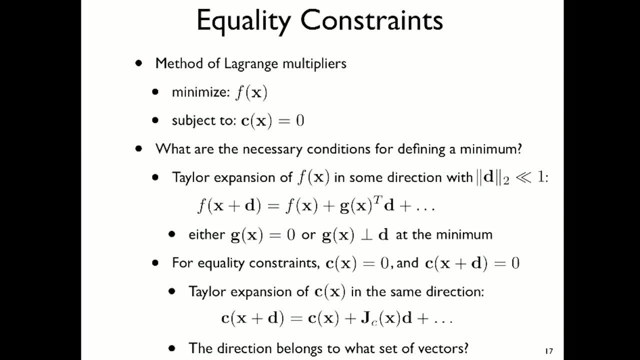 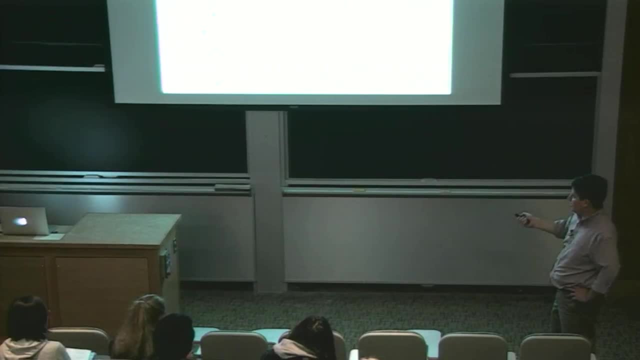 of c of x plus d about x. right, you'll get c of x plus d plus the Jacobian of c, right, all the partial derivatives of c with respect to x multiplied by d. We know that c of x plus d is zero and c of x is zero. 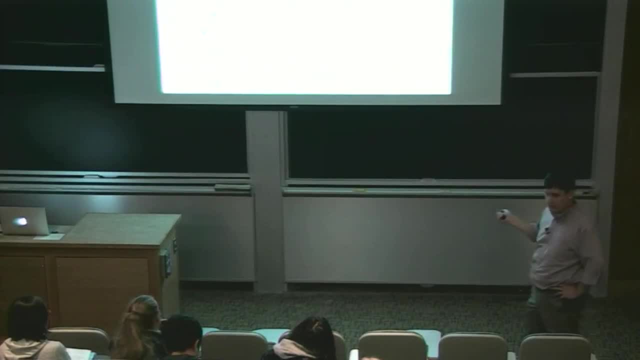 So the directions d belong to what set of vectors? The null space, right? So these directions have to live in the null space of the Jacobian of c. okay, So I can't step in any direction. I have to step in directions that are in the null space of c. 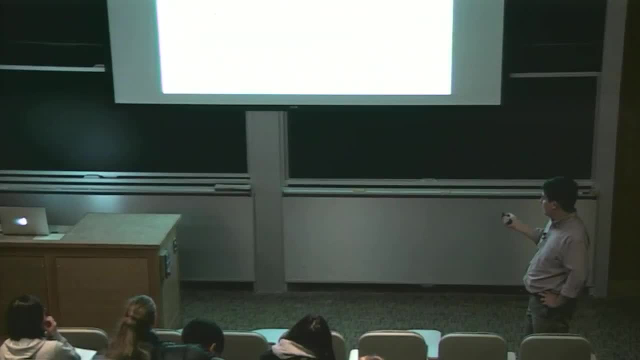 g is perpendicular to d as well, and d belongs to the null space of c. In fact, you know that d is perpendicular to each of the rows, But the null space is perpendicular to the rows of the Jacobian right. You know that. 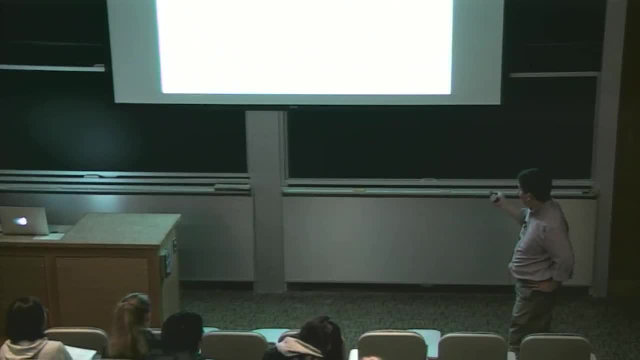 I just do the matrix vector product right, And so each element of this matrix vector product is the dot product of d, with a different row of the Jacobian. So those rows are a set of vectors, okay. Those rows describe the range of j transpose, okay. 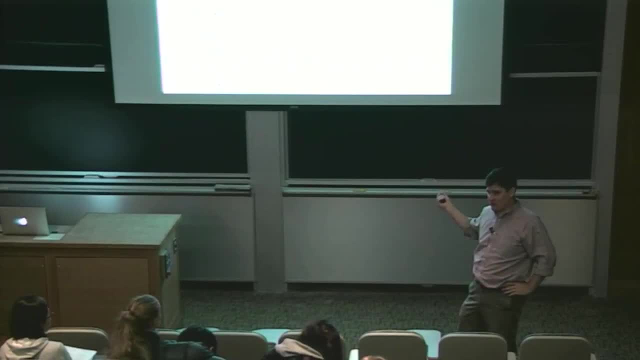 or the row space of j subspaces, and I said we almost never use those other ones, but this is one time when we will, So those rows belong to the range of J transpose where they belong to the left null space of J. I need to find a G a gradient which is 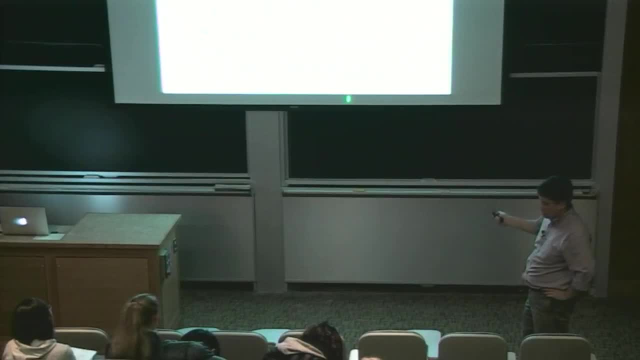 always perpendicular to D, and I know D is always perpendicular to the rows of J, So I can write G as a linear superposition of the rows of J. As long as G is a linear superposition of the rows, it'll always be perpendicular. 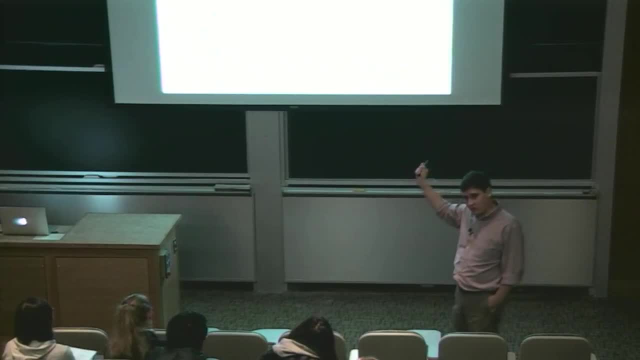 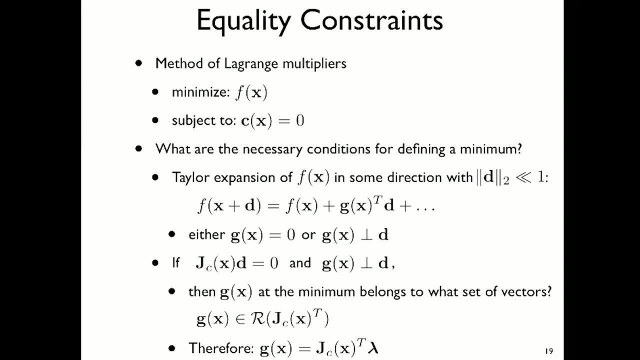 to D. Vectors from the null space of a matrix are orthogonal to vectors from the row space of that matrix, it turns out, and they're orthogonal for this reason. So it tells us, if JD is zero, then D belongs to the null space. G is perpendicular to. 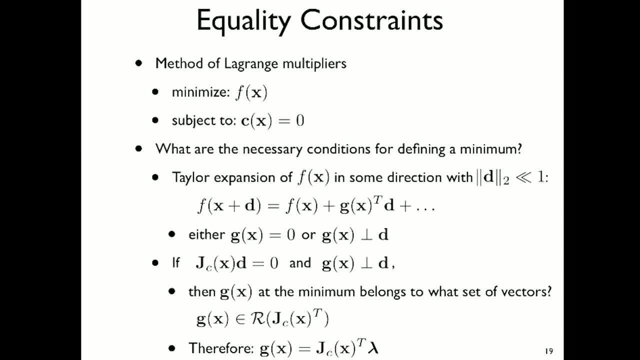 to D. That means I could write G as a linear superposition of the rows of J. So G belongs to the range of J transpose, or it belongs to the row space of J. Those are equivalent statements And therefore I should be able to write: 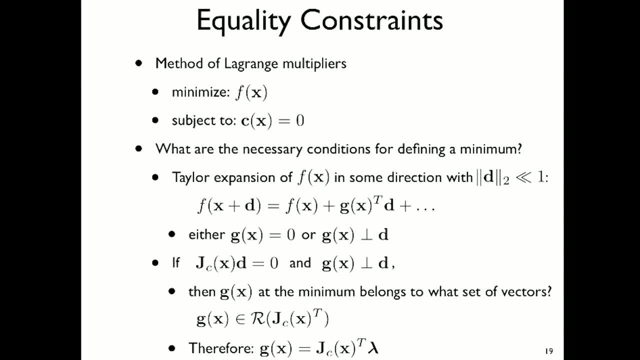 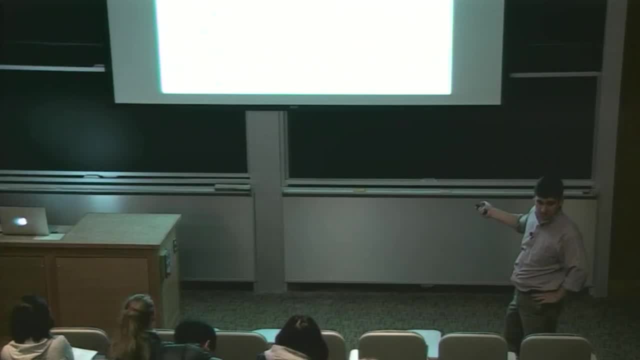 G as a linear superposition of the rows of J, And one way to say that is: I should be able to write G as J transpose times some other vector, lambda. That's an equivalent way of saying that G is a linear superposition of the rows of J. 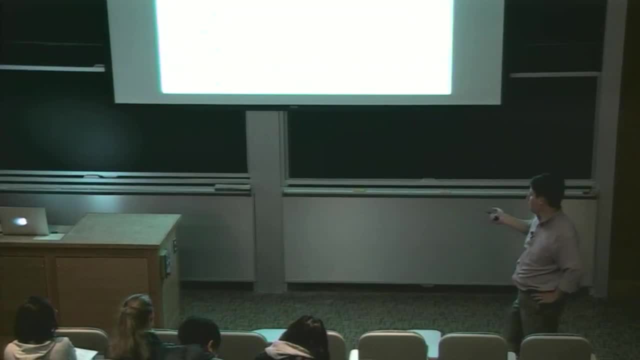 I don't know the values of lambda, So I introduced a new set of unknowns, a set of Lagrange multipliers. My minima is going to be found when I satisfy this equation, just like before, and when I'm able to satisfy. 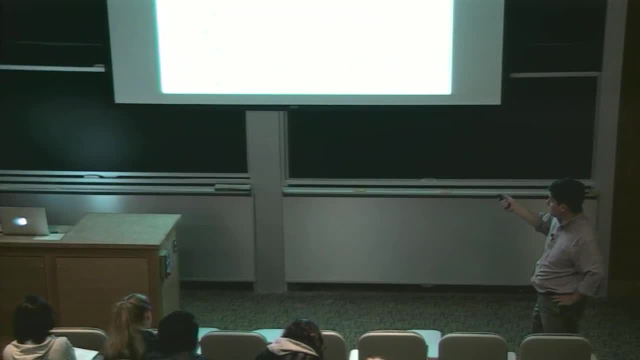 all of the equality constraints. So how many Lagrange multipliers do I have here? Can you figure that out? You can talk with your neighbors if you want. Take a couple of minutes, Tell me how many Lagrange multipliers, how many elements. 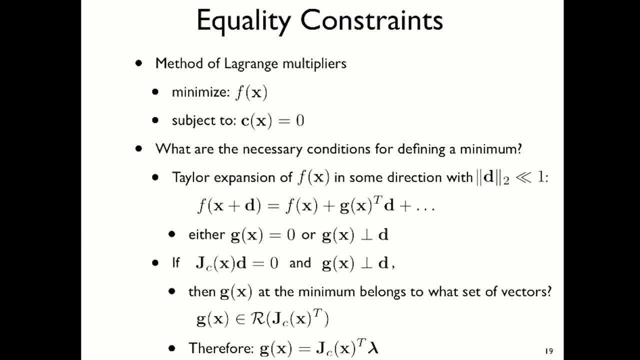 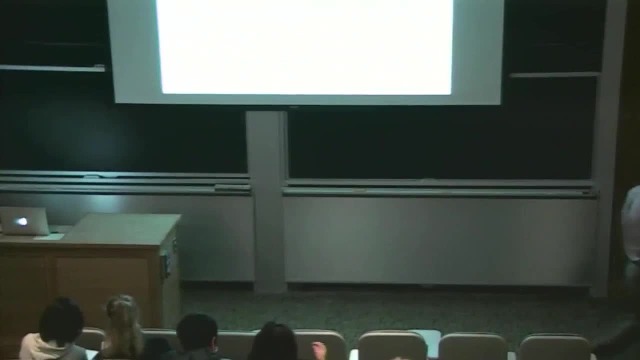 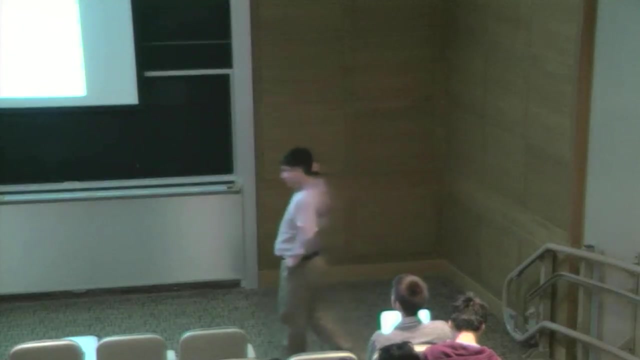 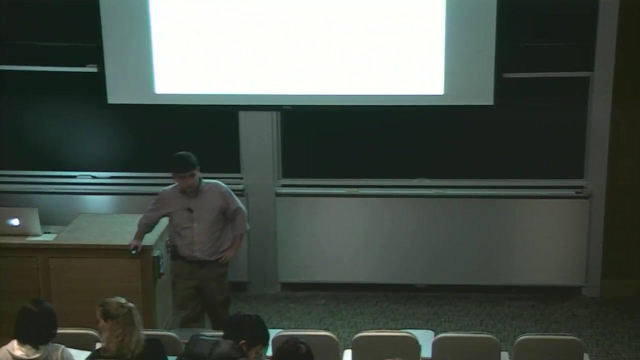 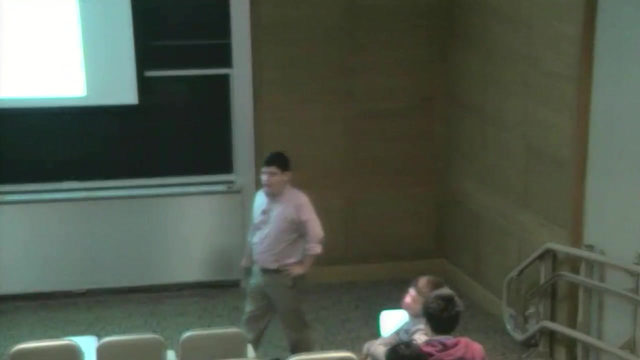 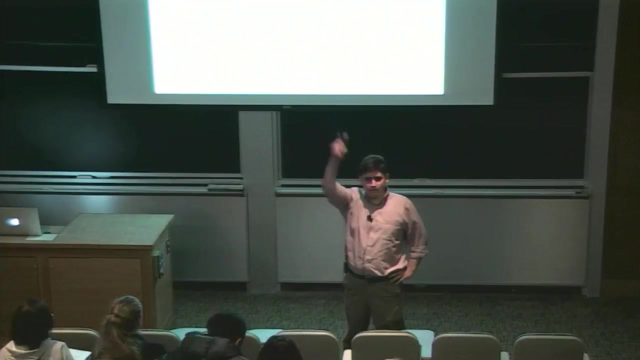 are in this vector? lambda? How many? How many elements are in lambda? Can you tell me, Sam? Yes, It's the same as the number of equality constraints. J came from the gradient of C. It's the Jacobian of C. 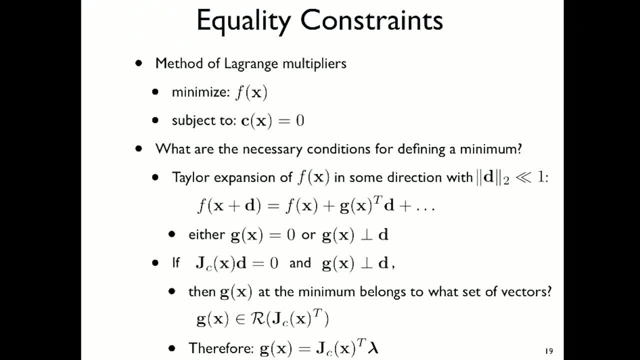 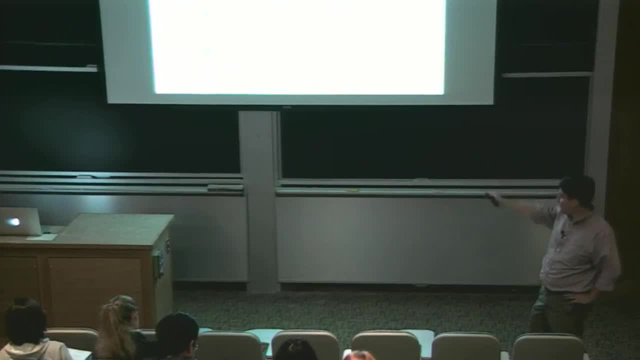 So it has a number of columns equal to the number of elements in X. because I'm taking partial derivatives with respect to each element of X, It has a number of rows equal to the number of elements of C. So J transpose, I just transpose those dimensions. 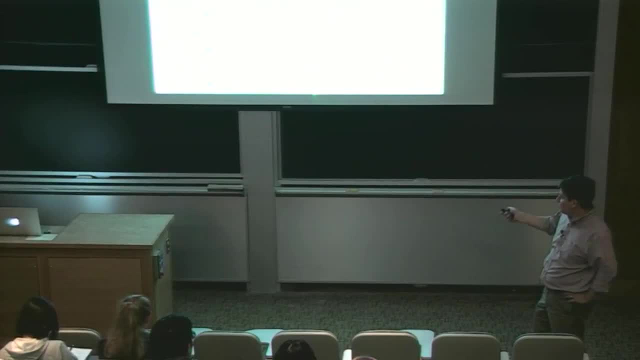 And lambda must have the same number of elements as C does in order to make this product make sense. So I introduce a new number of unknowns. It's equal to exactly The number of equality constraints that I had, Which is good, because I'm going to make a system of equations. 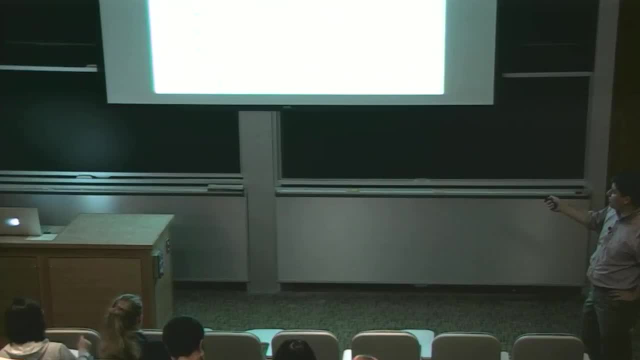 that says G of X minus J, transpose lambda equals 0 and C of X equals 0. And the number of equations here is the number of elements in X for this gradient and the number of elements in C for C, And the number of unknowns is the number of elements in X. 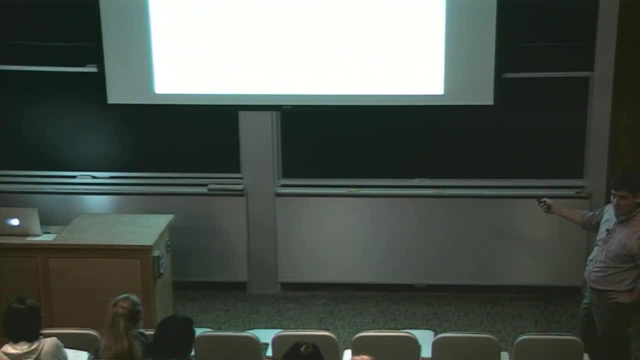 and the number of elements in C associated with the Lagrange multiplier. So I have enough equations and unknowns. So I have enough unknowns to determine all of these things. So whether I have one equality constraint or a million equality constraints, the problem is identical. 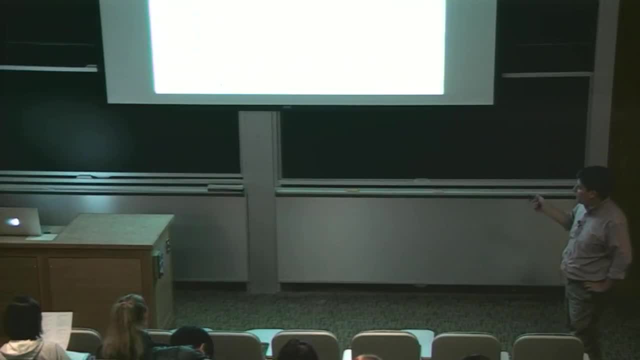 We use the method of Lagrange multipliers, We have to solve an augmented system of equations for X and this projection on the row space of J, which tells us how the gradient is stretched or composed of elements of the row space of J. These are the conditions associated. 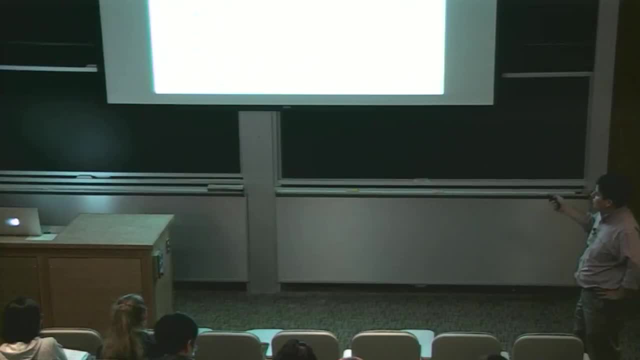 These are the conditions associated with a minima in our objective function on this boundary dictated by the equality constraint. And, of course, the solution set is a critical point of a Lagrangian which is F of X minus C dot lambda, And it's not a minimum of it. 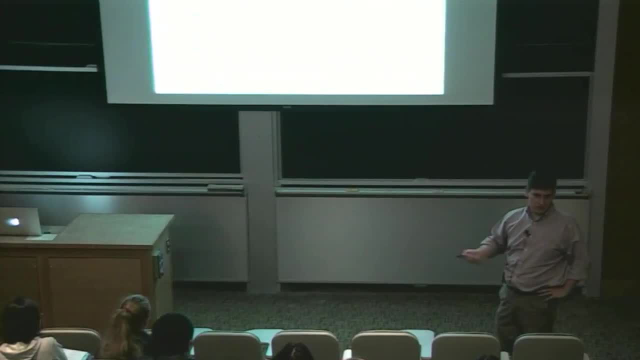 It's a critical point, It's a saddle point, it turns out of this Lagrangian. So we got to check: Did we find a saddle point or not? when we find a solution to this equation here, OK, OK, OK. 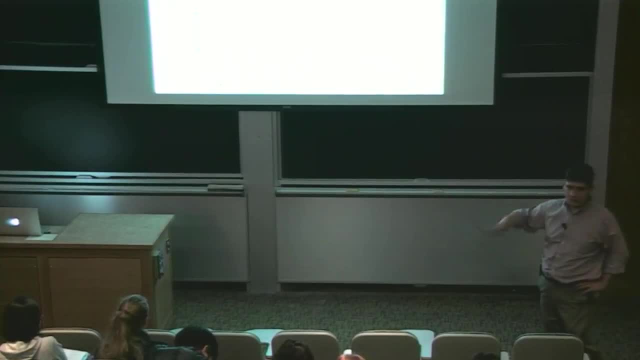 But it's just a system of nonlinear equations. If we have some good initial guess, what do we apply? Newton-Raphson right Converge rate towards the solution. If we don't have a good initial guess, well you know. 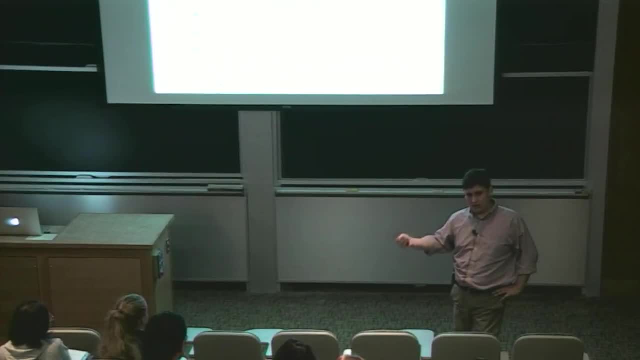 we've discussed lots of methods we could employ, like homotopy or continuation, to try to develop good initial guesses for what the solution should be. Are there any questions about this? Good, OK, So this is. you know, You go to MATLAB and you call fmincon, right. 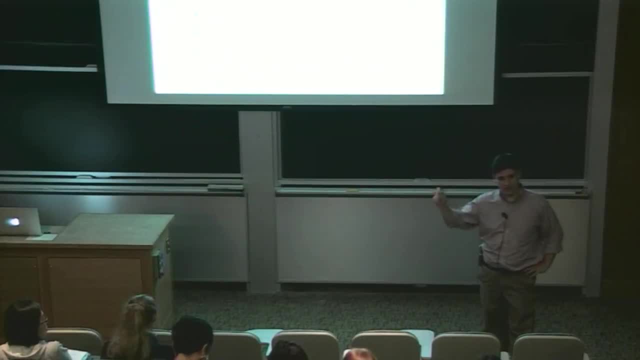 Do a minimization problem and you give it some constraints- Linear constraints, nonlinear constraints, It doesn't matter actually, right, The problem is the same for both of them. It's just a little bit easier if I have linear constraints, OK. 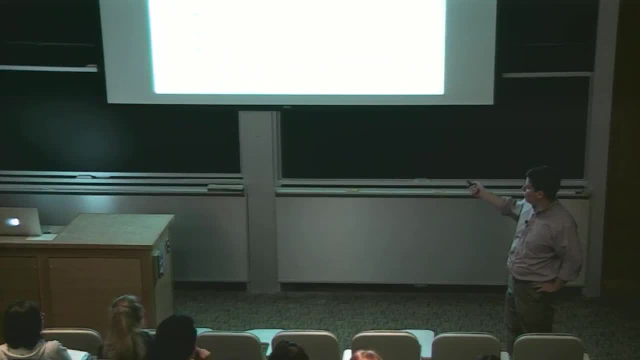 If this constraining function is a linear function, then the Jacobian- I know it's the coefficient matrix of this linear problem. I only have to solve linear equations down here, So the problem is a little bit simpler to solve, OK. 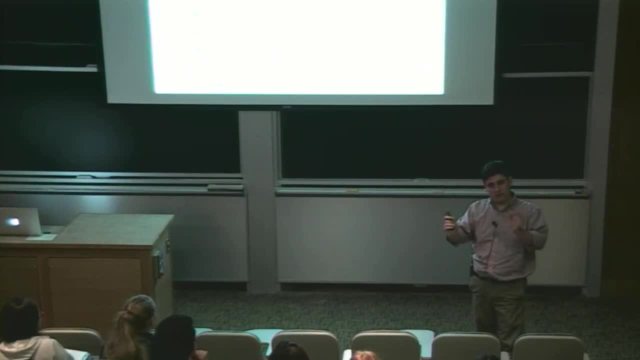 So MATLAB sort of breaks these apart so it can use different techniques depending on which one which sort of problem is posed, But the solution method is the same. It does the method of Lagrange multipliers to find the solution. OK. 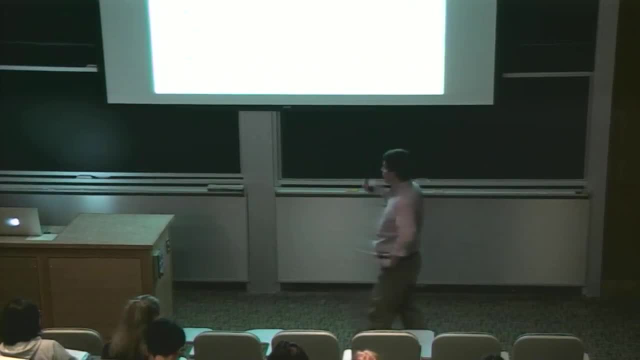 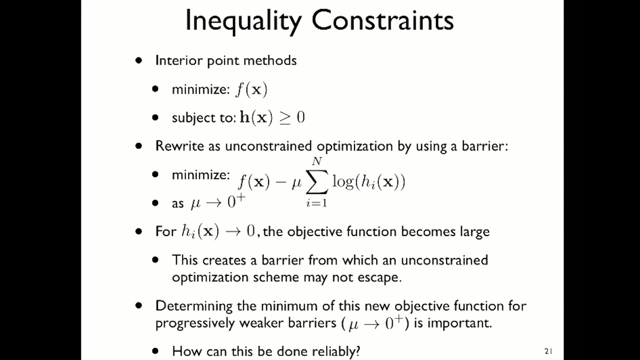 Inequality constraints. So interior point methods were mentioned And it turns out this is really the best way to go about solving generic inequality constrained problems. So these are problems of the sort right: Minimize f of x subject to h of x is positive, or at least not negative. 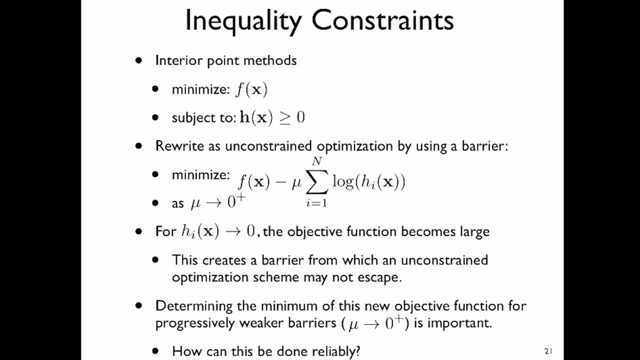 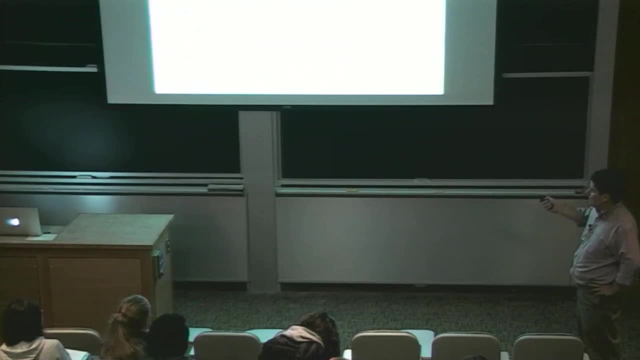 OK, This is some nonlinear inequality that describes some domain and its boundary in which the solution has to live, And what's done is to rewrite as an unconstrained optimization problem with a barrier that's incorporated. OK, This looks a lot like the penalty method, but it's very different. 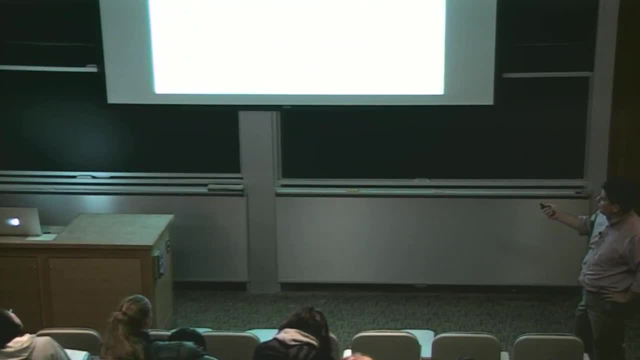 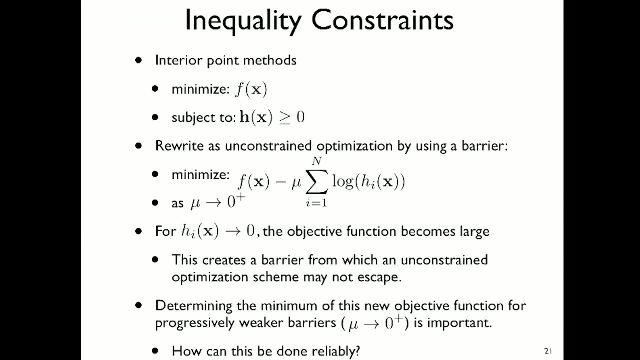 And I'll explain how Right. So instead we want to minimize this f of x minus mu times the sum of log of h. each of these constraints, OK. If h is negative, OK, the log will be. we'll take the log of the negative argument, OK. 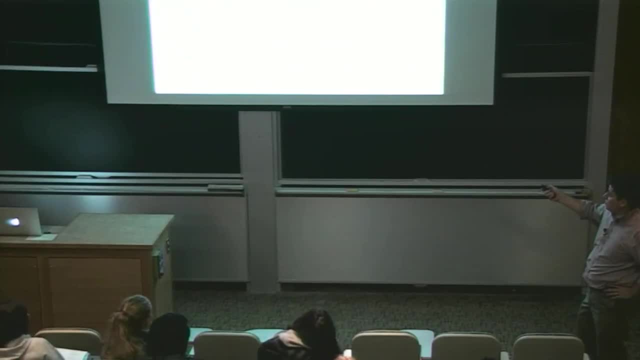 That's a problem computationally. So the best we could do is approach the boundary where h is equal to 0, right. And as h goes to 0, the log goes to minus infinity. So this term tends to Blow up because I got a minus sign in front of it, right? 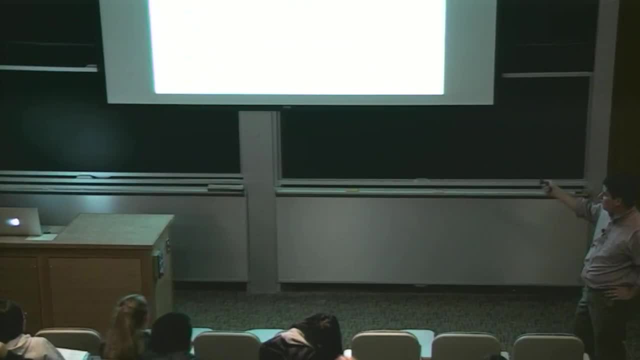 So this is sort of like a penalty, OK, But it's a little different because the factor in front- I'm actually going to take the limit as mu goes to 0,. OK, I'm going to take the limit as this factor gets small. 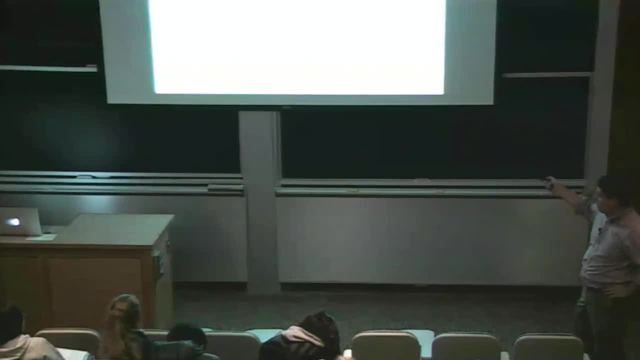 rather than gets big. OK, The log will always get big as I approach the boundary of the domain. right, It'll blow up. OK, So that's not a problem. But I can take the limit that mu gets smaller and smaller. 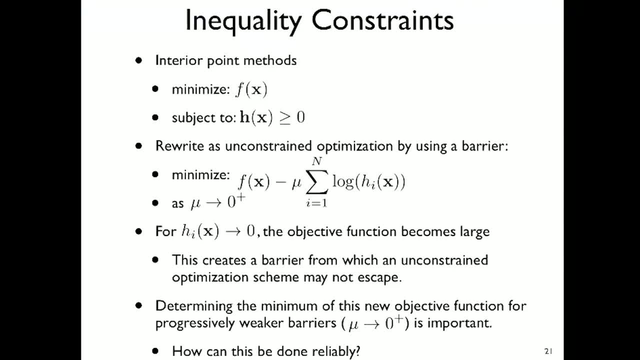 And this quantity here will have less and less of an impact on the shape of this new objective function. as mu gets smaller and smaller, right The impact will only be nearest the boundary. Does that make sense? So you take the limit that mu approaches 0.. 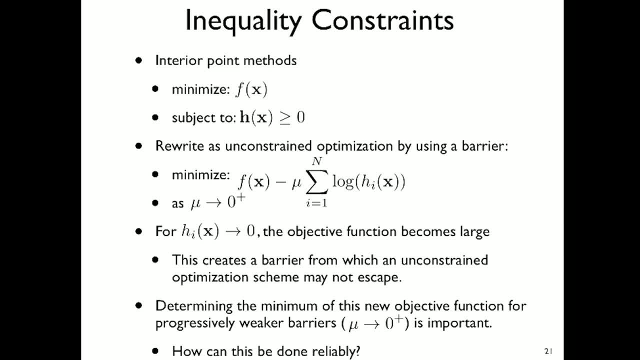 It's got to approach it from the positive side, not the negative side, so everything behaves well. OK, This is called an interior point method, So we have to determine the minimum of this new objective function for progressive, progressively weaker barriers. OK, 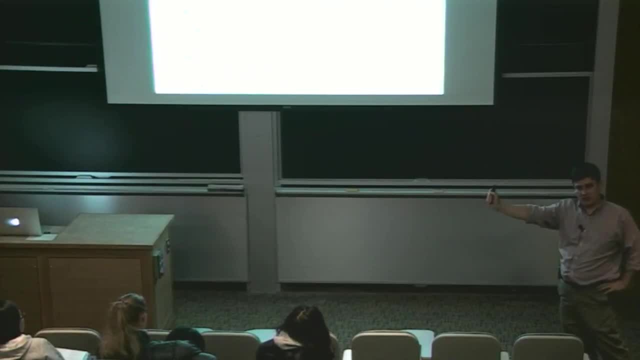 So we might start with some value of mu and we might reduce mu progressively right until we get mu down small enough that we think we've converged to a solution. So how do you do that reliably? What's the procedure one uses to solve a problem successively? 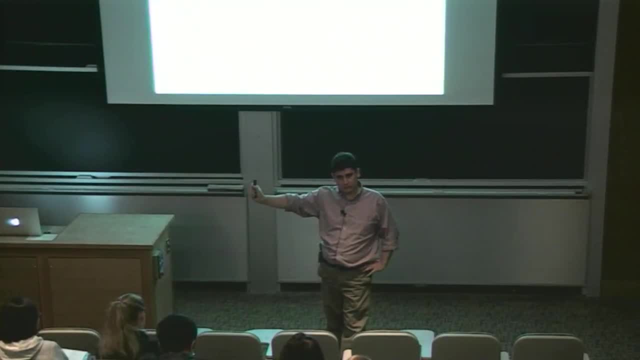 for different parameter values. Yeah, it's a homotopy, right? You're just going to change the value of this barrier parameter, Right? And you're going to find a minimum If you make a small change in the barrier parameter. 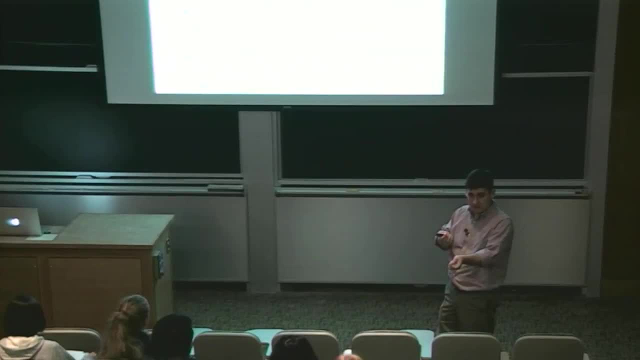 that's going to serve as an excellent initial guess for the next value, right? And so you're just going to take these small steps right, And the optimization routine is going to carry you towards the minimum in the limit that mu goes to 0.. 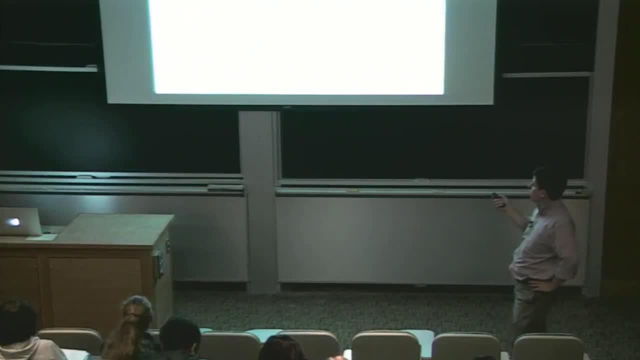 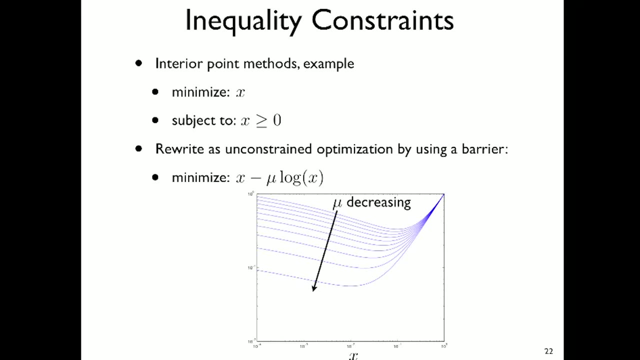 So you do this with homotopy. Here's an example of this sort of interior point method, a trivial example: right Minimize x subject to x being positive. So we know the solution lives where x equals 0. But let's write this as unconstrained optimization. 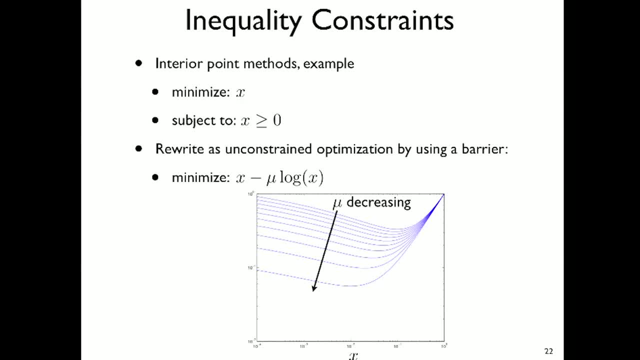 using a barrier. So minimize x minus mu times log x. Here's x minus mu times log x. So out here, where x is big, x wins over log x. So everything starts to look linear. But as x becomes smaller and smaller, 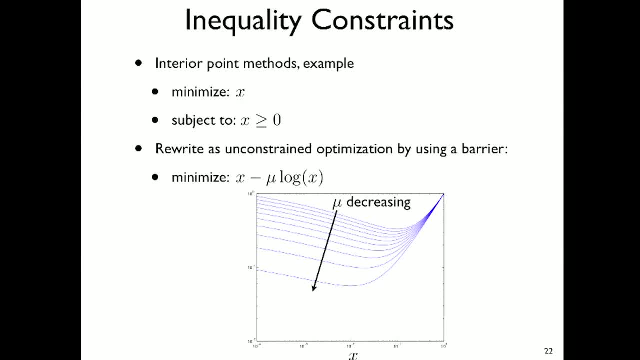 log x gets very negative. So minus log x gets very positive. And here's the log creeping back up. And as I decrease mu, smaller and smaller. you can see the minimum. This function is moving closer and closer and closer to 0.. 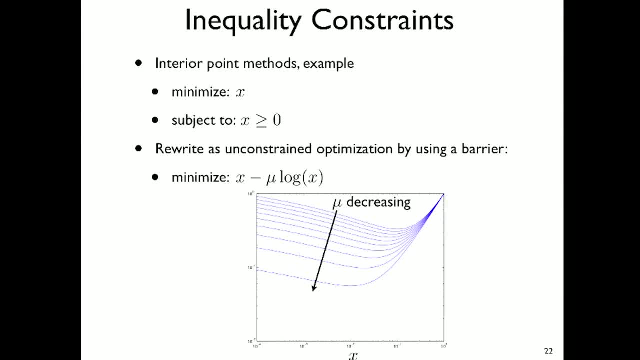 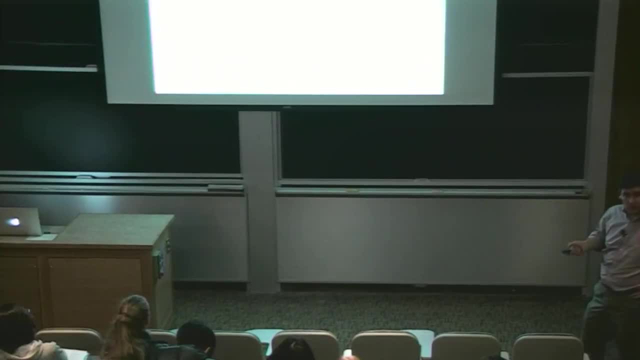 So if I take the limit, that mu decreases from some positive number towards 0, eventually this minimum is going to converge to the minimum of the inequality-constrained optimization problem. Make sense, OK? OK, so we want to do this. You can choose any barrier function you want. 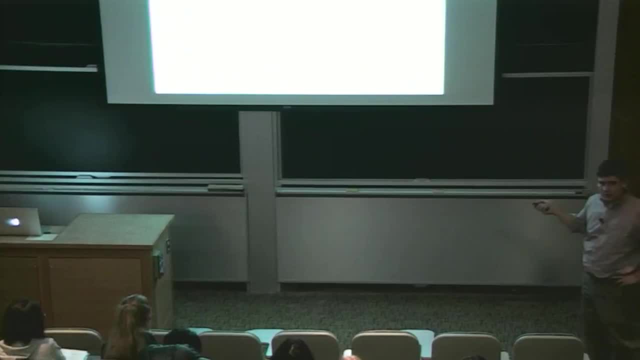 Any thoughts on why a logarithmic Barrier is used? No, OK, That's OK. So minus log is going to be convex. Log isn't convex, But minus log is going to be convex, So that's good, It's going to if this function is convex. 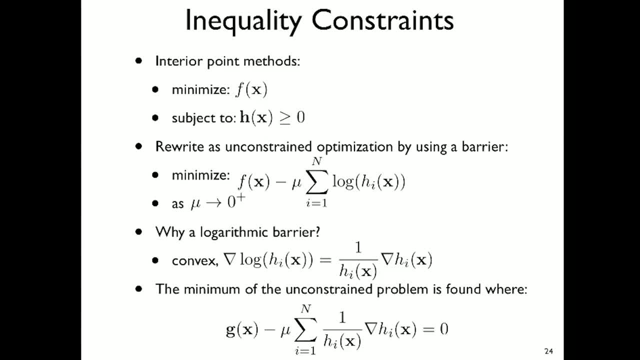 then their combination is going to be convex and will be OK. But the gradient of the log is easy to compute, right? Grad log h is 1 over h, grad h, right? So if I know h, I know grad h. It's easy for me to compute the gradient of log h. 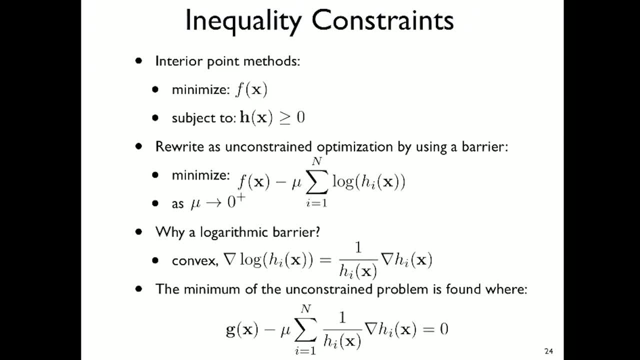 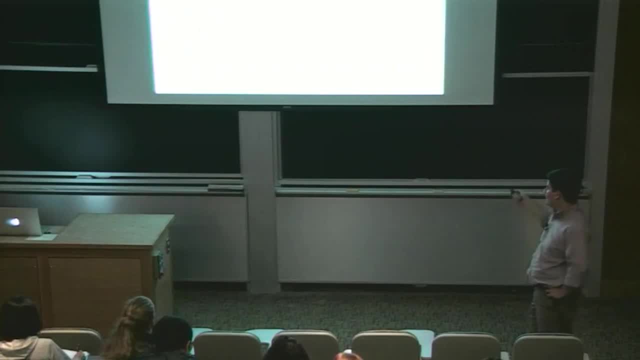 We know we're going to solve this unconstrained optimization problem where we need to take grad of the subjective function equals 0. So the calculations are easy. right, The log makes it easy like that. The log is also like the most weakly singular function. 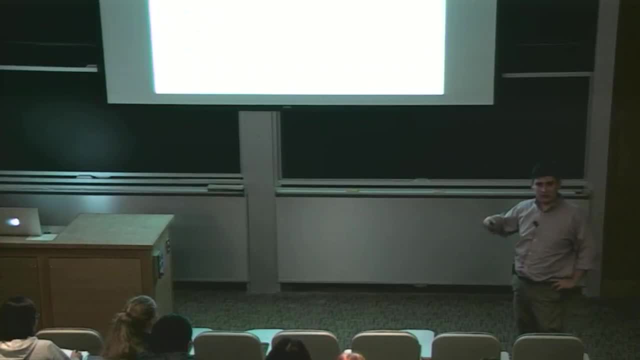 available to us right Out of all the toolbox, of all problems we can reach to, the log has sort of the mildest sort of singularities. Singularities at both ends, which is sort of funny, But the mildest sort of singularities. 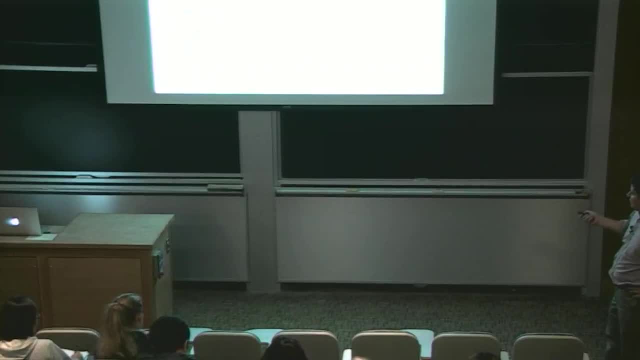 you have to cope with. OK, So we want to find the minimum of these unconstrained optimization problems where the gradient of f minus mu sum 1 over h. grad h is equal to 0. And we just do that for progressively smaller values of mu and we'll converge to a solution. 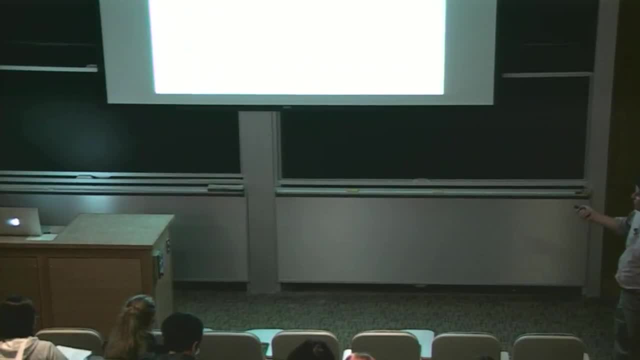 That's the interior point method. You use homotopy to study a sequence of barrier parameters, or continuation to study a sequence of barrier parameters. You stop the homotopy. You stop the homotopy or continuation. when, what? How are you going to stop? 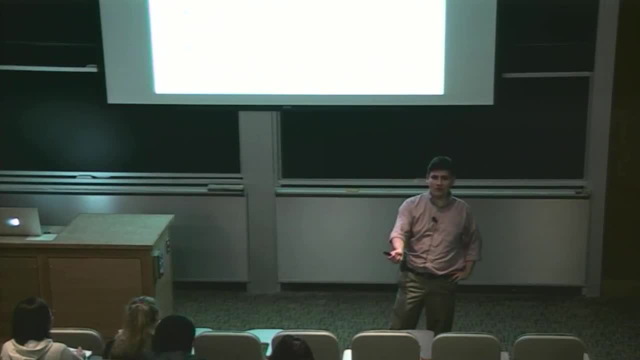 I've got to make mu small. right, I want to go towards the limit. mu equals 0.. I can't actually get to. mu equals 0, right, I just got to approach it. So how small do I need to make mu before I quit? 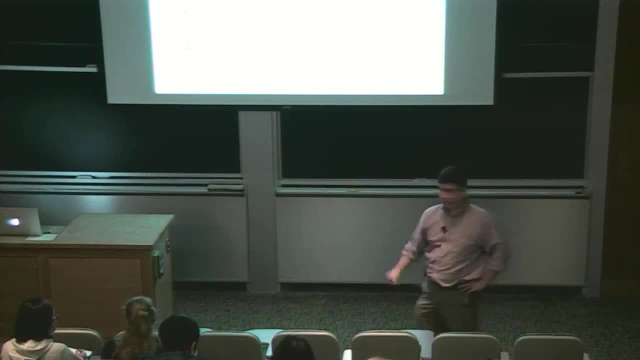 It's an interesting question. What do you think? I'll take this answer first. So I said, well, it doesn't affect your. Oh, good, So we might look at the solution And see: is the solution becoming less and less sensitive to the choice of mu? 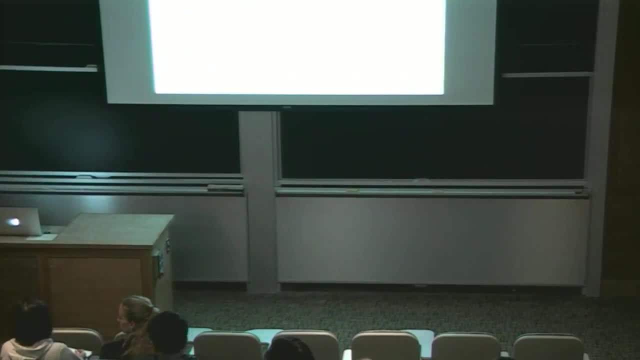 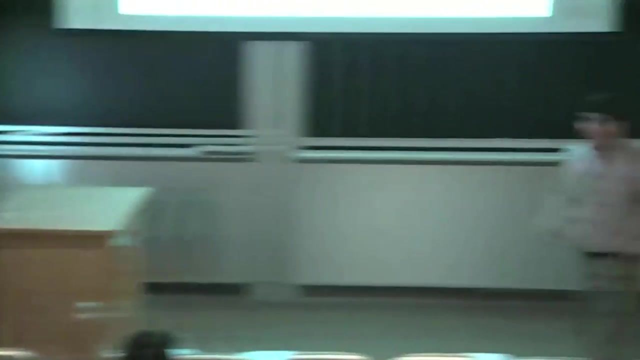 Good. Did you have another suggestion? Look, a set of tolerance, right? OK, You could change Mm-hmm Right, right, right, right, So you Good. So there were two suggestions here. One is along the lines of a step norm criteria, right. 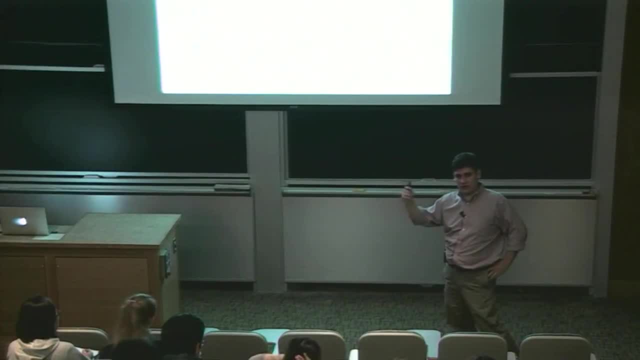 Like I check my solution as I change mu and I ask: when does my solution seem relatively insensitive to mu? right, When the changes in these steps relative to mu get sufficiently small, I might be willing to accept these solutions as reasonable solutions for the constrained optimization. 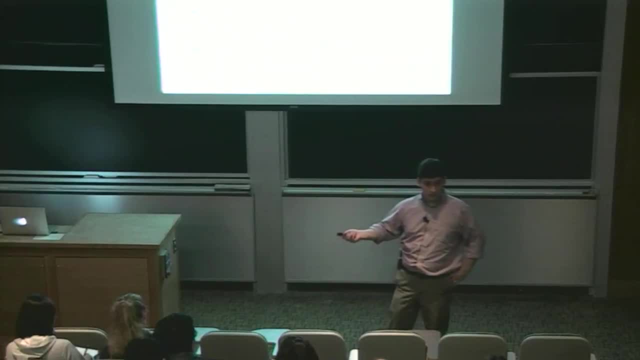 I can also go back and I can check sort of function norm criteria right, I can take the value of x I found as the minimum and I can ask how good a job does it do satisfying the original equations? OK, How far away am I from satisfying the inequality? 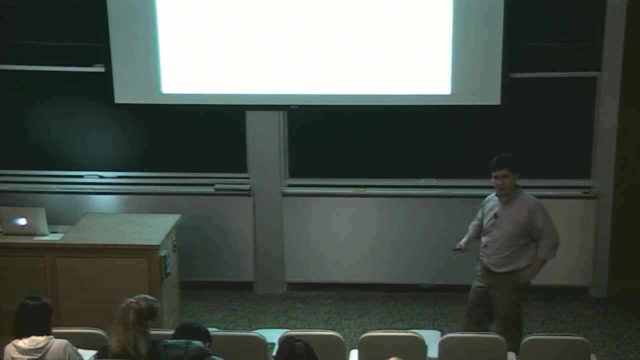 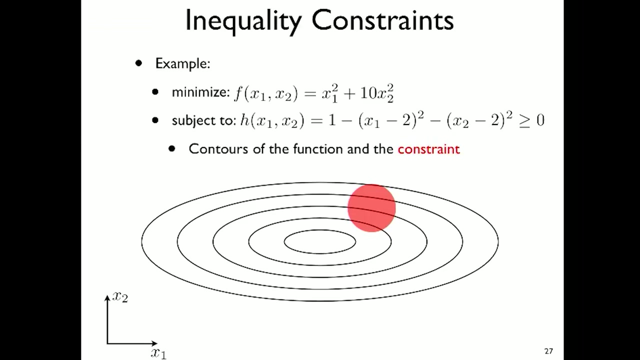 constraint. How close am I to actually minimizing the function within that domain? OK, So we're running out of time here. Let me provide you with an example, So let's minimize again. I always pick this function because it's easy to visualize, right? 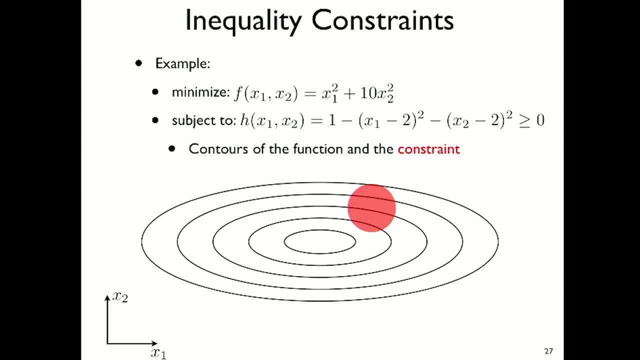 A nice parabolic function. It opens upwards And let's minimize its subject to the constraint right. So let's make that h of x1 and x2 is equal to 1 minus. well, the equation for a circle of radius 1,. 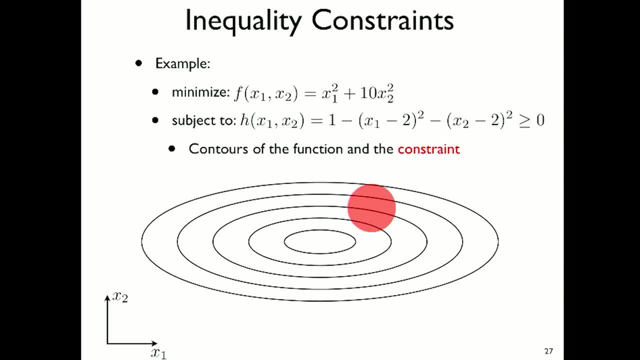 essentially the interior of that circle. OK, So here's the contours of the function and this red domain is the constraint, And we want to know the smallest value of f that lives in this domain. So here's some MATLAB code. You can try it out. 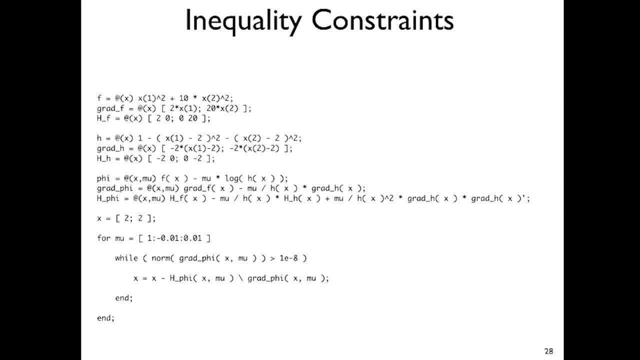 I make a function, the objective function, f. It's x squared plus 10x. OK, So x1 squared plus 10x2 squared. Here's the gradient, Here's the Hessian. Here I calculate h. Here's the gradient in h. 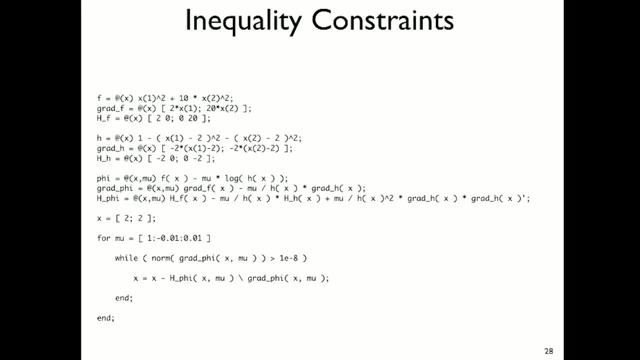 Here's the Hessian. in h I get to define a new objective function, phi, which is f minus mu, log h. This is the gradient in phi and this is the Hessian of phi. Oh man, what a mess. But actually not such a mess, because the log. 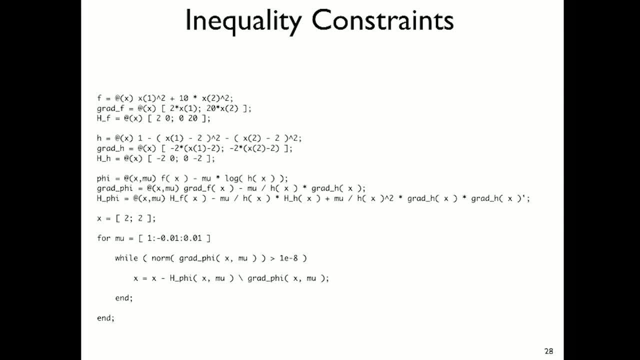 makes it really easy to take these derivatives. So it's just a lot of value, a lot of differential sort of calculus involved in working this out. But this is the Hessian of phi And then I need some initial guess, So I pick the center of my circle. 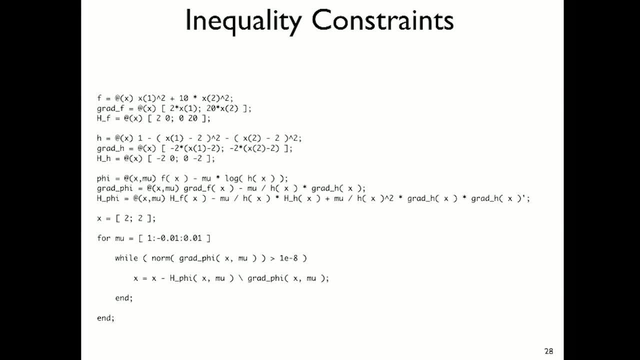 as an initial guess for the solution, And I'm going to loop over values of mu that get progressively smaller. I'll just go down to 10, to the minus 2, and stop for illustration purposes here, But really we should be checking the solution. 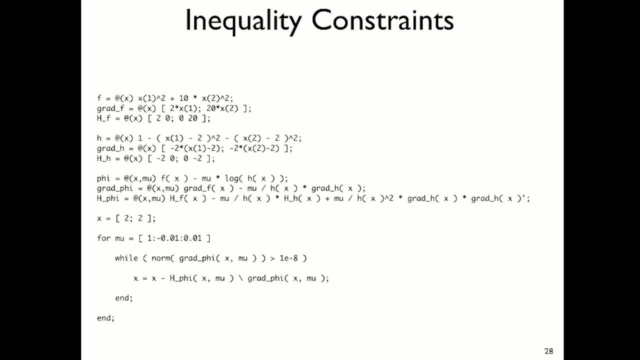 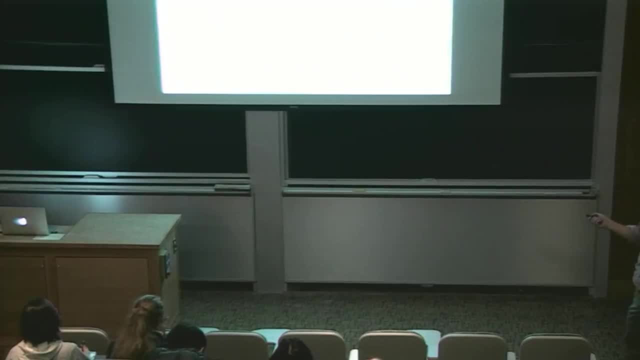 as we go and deciding what values we want to stop with. OK, And then this loop here: What's this do, What's it do? Can you tell What's that? Yeah, it's Newton-Raphson, right. x is x minus Hessian inverse times, grad phi, right. 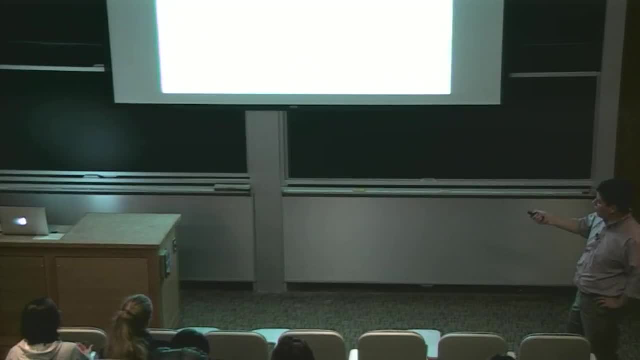 So I just do Newton-Raphson, I take my initial guess and I loop around with Newton-Raphson And when this loop finishes I reduce mu and it'll just use my previous guess as the initial guess for the next value of the loop. 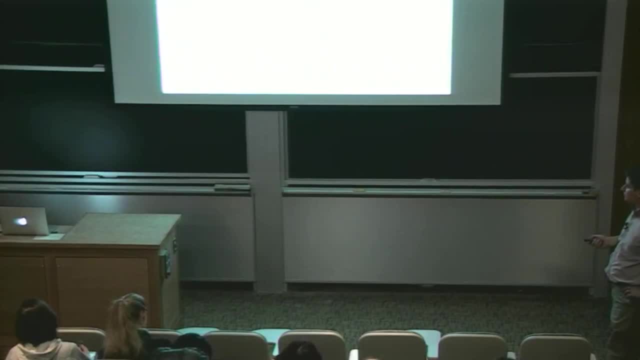 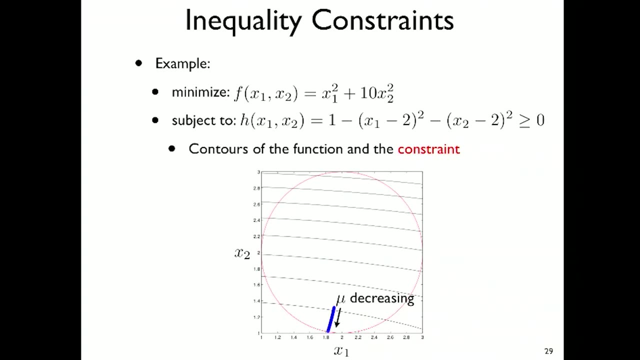 And that's what I'm going to do until mu is sufficiently small. OK, Interior point method. Here's what that solution path looks like. So mu started at 1, and the barrier was here. It was close to the edge of the circle, but not quite on it. 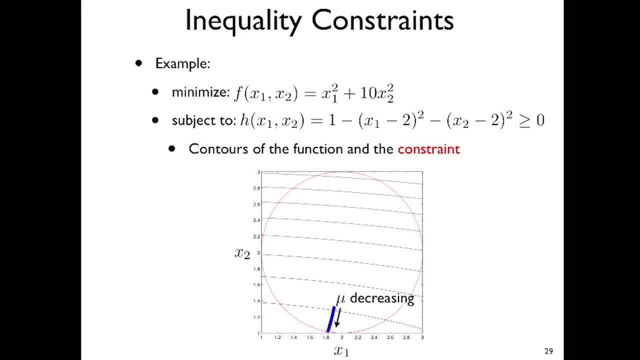 But as I reduced mu further and further and further, you can see the path, the solution path that was followed works its way closer to the boundary of the circle And the minimum is found right here. So it turns out the minimum of this function. 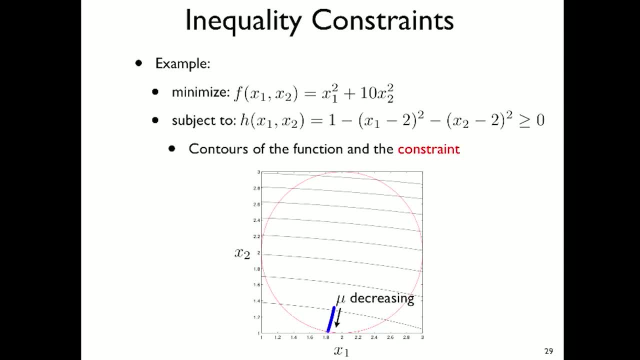 doesn't live in the domain. It lives on the boundary of the domain. OK, OK, OK. So we found that this point should be a point where the boundary of the domain is parallel to the contours of the function, since actually we didn't need the inequality constraint here. 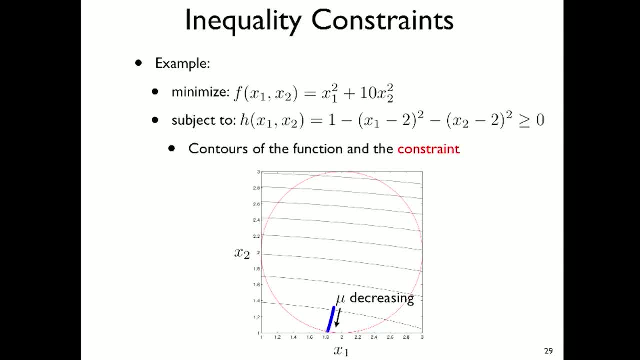 We could have used the equality constraint. The equality constraint problem has the same solution as the inequality constraint problem. And look, that actually happened. Here's the contours of the function. The contour of the function runs right along here And you can see it looks like it's. 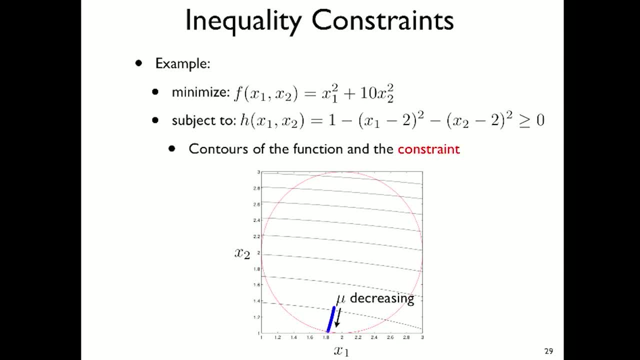 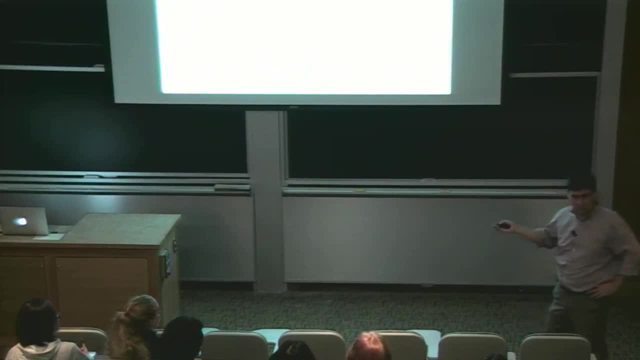 going to be tangent to the circle at this point. So the interior point method actually solved an equality constraint. So that's the inequality constraint problem in addition to an inequality constraint problem, which is sort of cool that you can do it that way. How about if I want to do a combination of equality? 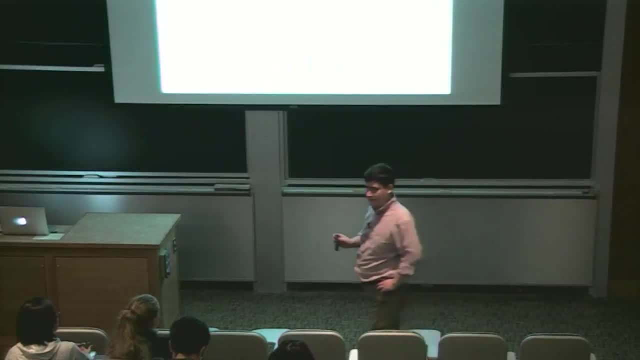 and inequality constraints. Then what do I do? Yeah, So you can convert the equality constraint into a problem. ADAM BERGSTRAM-, Perfect Right, Convert the equality constraint into and then do the interior point method on the Lagrange. 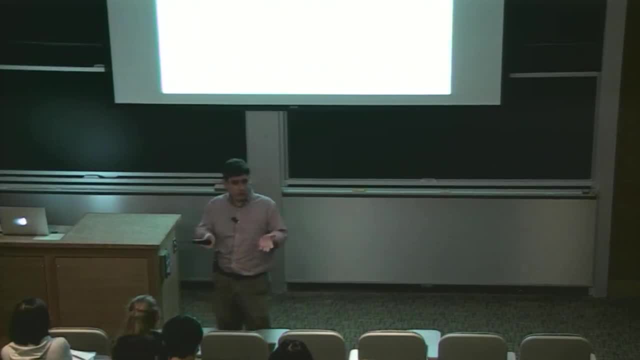 multiplier problem. OK, Now you've got a combination of equality and inequality constraint. This is exactly what MATLAB does. OK, So it converts equality constraints into Lagrange multipliers. Inequality constraints it actually solves using interior point methods Buried in that interior point method. 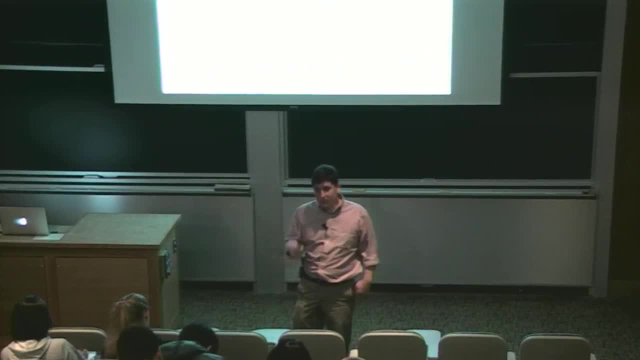 is some form of Newton-Raphson and steepest descent combined together like dogleg We talked about for unconstrained constraints, but it's also a way to solve the interior point method. ADAM BERGSTRAM- Yeah, So it's going to solve all of these.